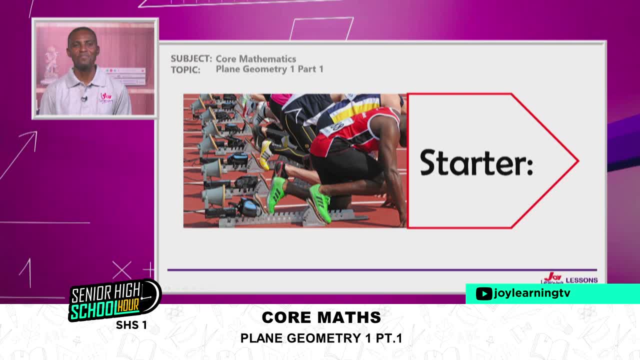 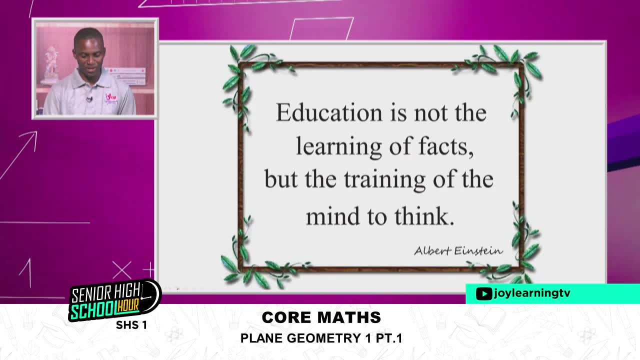 And as usual with our starters, And today our starters, The starter is going to be a motivational word. A motivational word, Something to think about, Something to prepare your mind as you learn and as you journey in your academic career. Education is not the learning of facts, but the training of the mind to think. 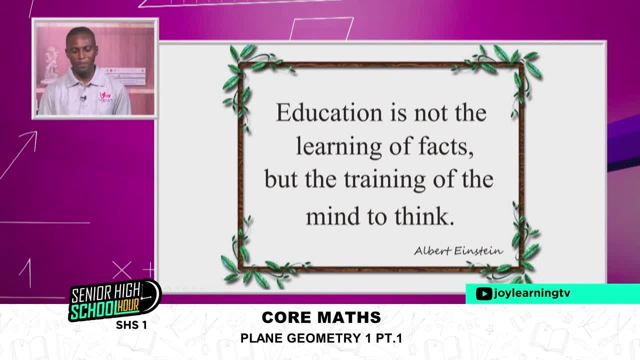 Education is not the learning of the facts, but training of the mind to think, Said by Albert Einstein. Whatever we are giving you in school is not just to memorize something, write exams and pass, and you say that is all. No, our aim is to prepare your mind so you can think and be creative, be innovative, be problem solver. 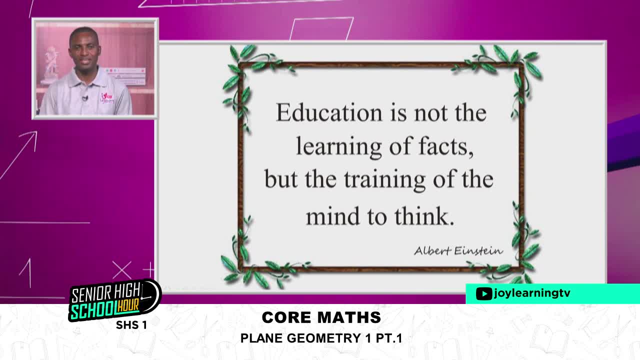 That is all about education, And mathematics does a lot in that direction. Mathematics is all about preparing you to build your thinking capability, to build analytical skills and to become more problem solver, more critical thinker. Mathematics is all about preparing you to build your thinking capability, to build analytical skills and to become more problem solver, more critical thinker. 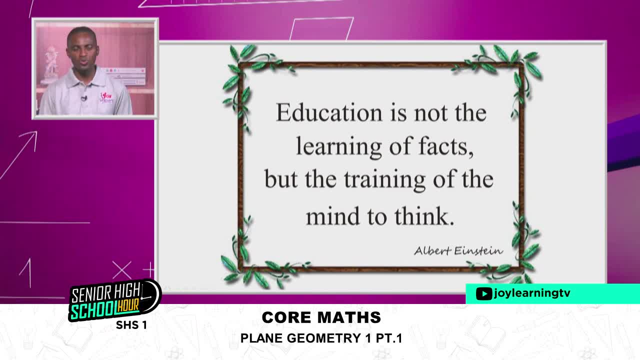 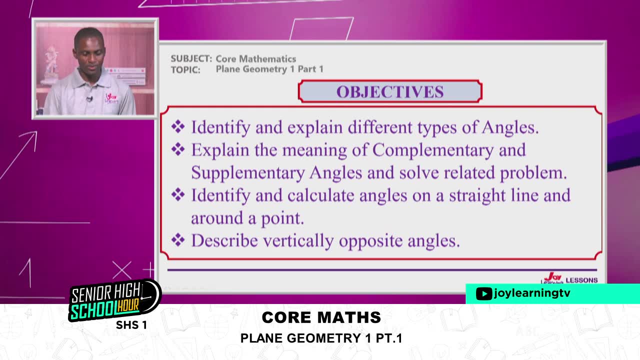 And an innovator. That is all we want you to do. so Don't learn for examination. learn for life. learn to build your capacity so that you can be the best You ought to be in the country. So for today, like you say, we are doing Plane Geometry 1, and we're dealing with Part 1, and for Part 1, today, we are going to handle the following objectives: 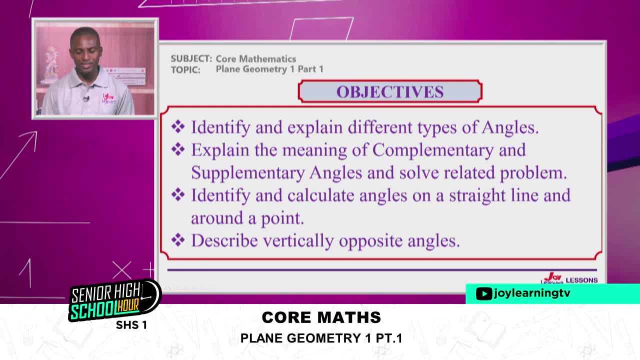 By the end of today's session, You should be able to Identify and explain Different types of angles, explain the meaning of complementary and supplementary angles and solve related problems that goes with them. then again, we are going to identify or, by the end of the lesson we'll be. 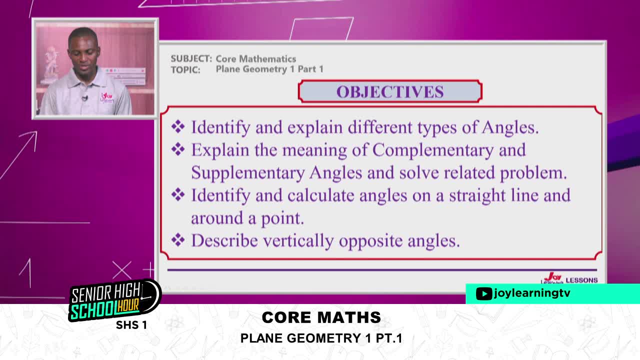 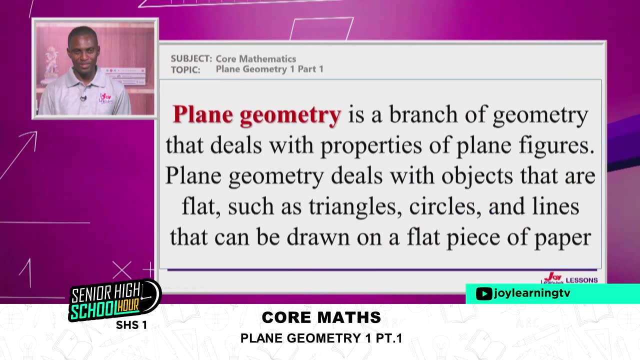 able to identify and calculate angles on a straight line and angles around a point, and then, if time permits us, we'll further go on to describe vertically opposite angles. so these are objectives, and we hope we'll be able to achieve all of them before we end today's lesson. so what? 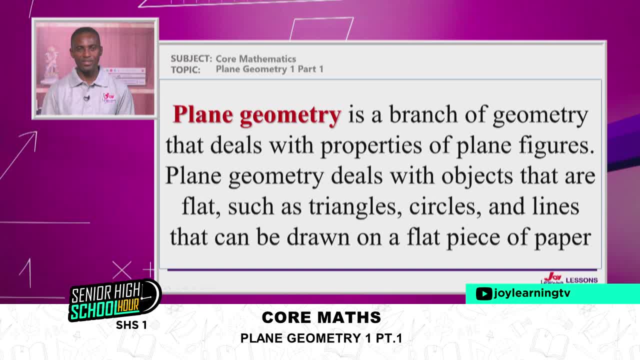 is plain geometry. what is it about? what are we going to learn as far as this topic is concerned? here we see. it is a branch of geometry that deals with properties of plain figures. a branch means geometry itself is a very big program, or let's say a course, and we are looking at only plain geometry. 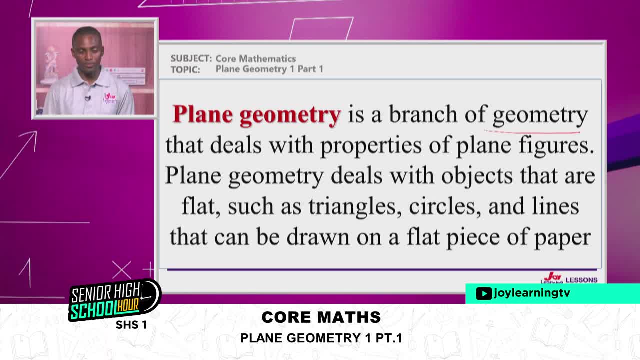 in few times. we're looking at solid geometry, and then we also have what you call coordinate geometry, and in some cases we also talk about analytical geometry, and so we are dealing with a aspect where we deal with objects that are flat, such as triangles, circles, lines that can be drawn. 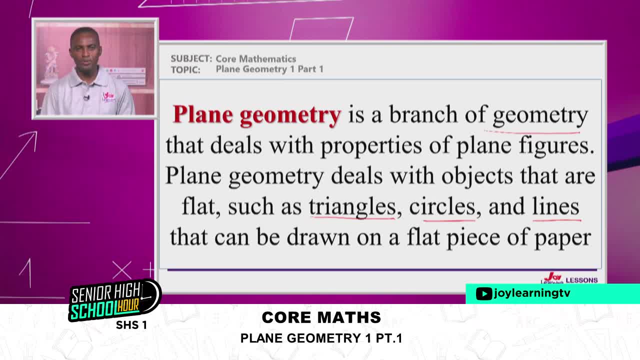 on a flat piece of paper, and so plain geometry is all about two dimensions, and no, we can't hold two dimensions. so we are going to talk about the, the square, the angles, the lines and so on and so forth. so talk of plane. yes, we have other shapes. 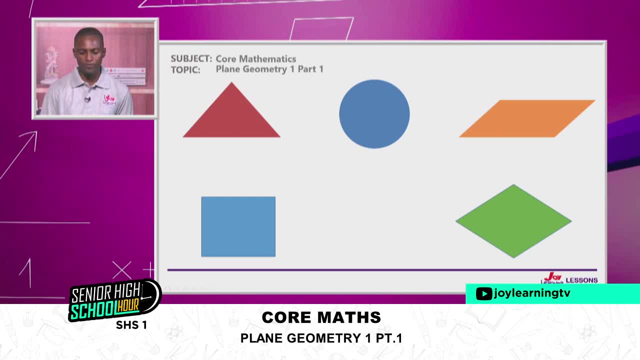 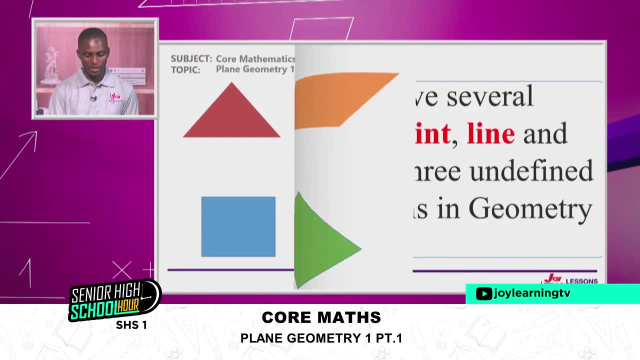 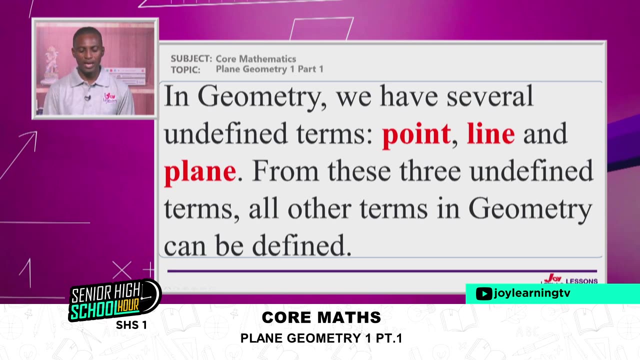 that are considered as plain, like triangle is a plain figure, circle is a plain figure, um, paragraph is a plain figure, we have a square plane figure, rhombus, and so on and so forth. right now in geometry we have several undefined terms, terms like point line and plane, but they're very 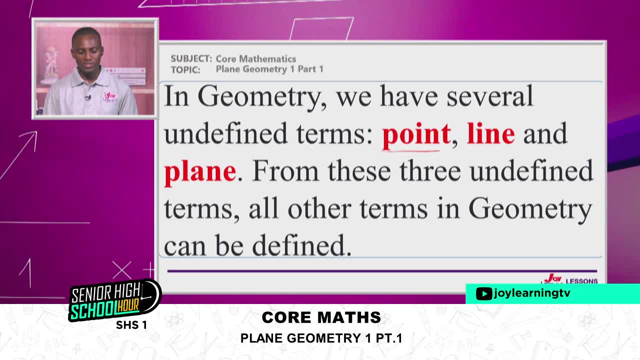 difficult to define. but then if you're able to define them, they will serve as the basis for other definitions. so from these three undefined terms, all other terms in geometry can be defined. all right. so we see that in all geometry it's all about point lines, plain angles and so on, and 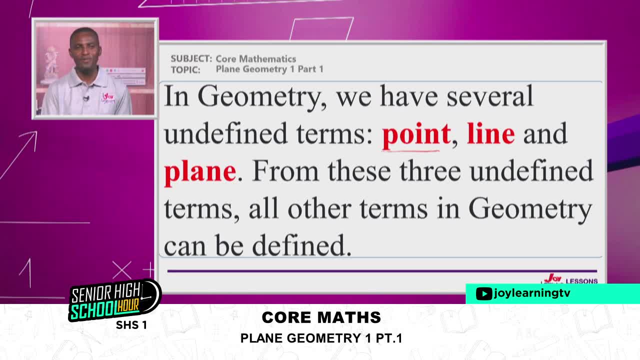 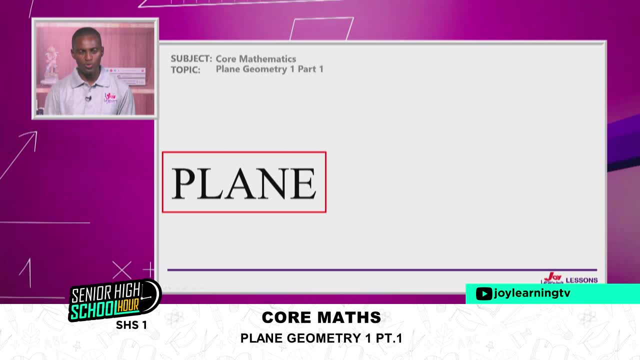 so forth. maybe with angles, it comes from the definition of a line or using line to define angles. so, based on these three, we can look at them. so we want to look at the one after the other, maybe talk about plane, what is plane? and topic itself is plain geometry. so when we say plane, what does? 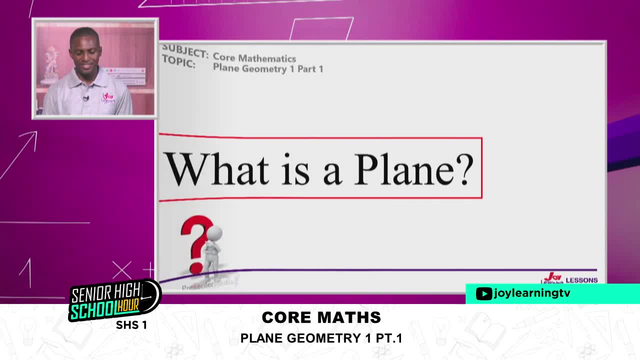 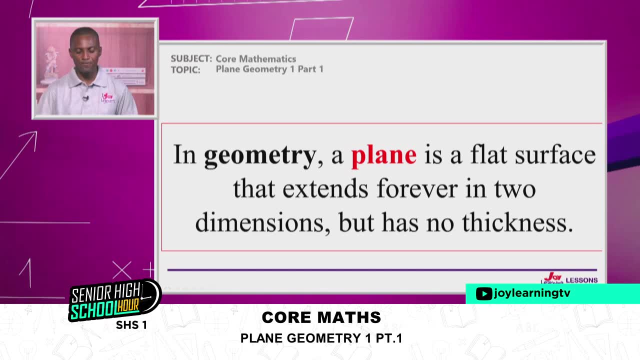 it mean all right. so by definition in geometry we are saying for plane it is a flat surface that extends forever in two dimensions but has no thickness. the moment it gets thickness then it means it will be a three dimension and so it has only two dimension. and it can be like this: 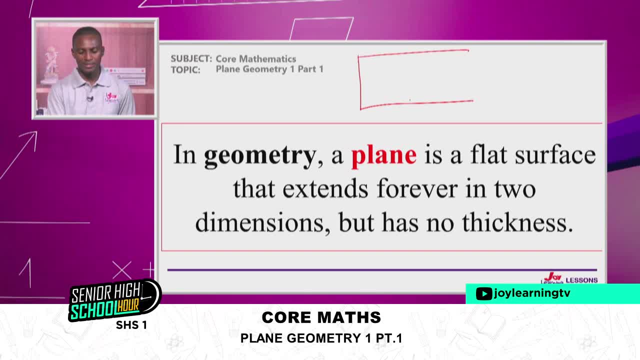 all like that. this is the same as this, so they move in the same direction- opposite direction, but this is also the same as that. so this two dimension is what we are referring to, but then if you're able to do something like this, then we get three dimension, so we can have this following: 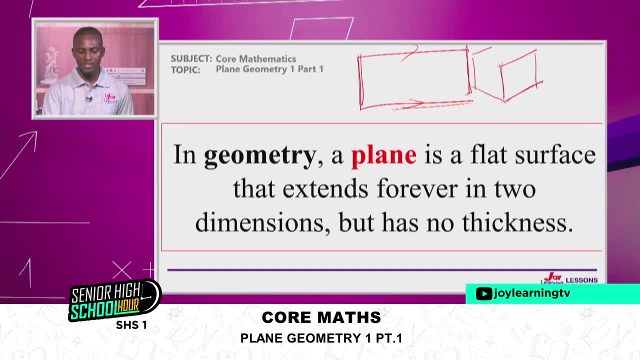 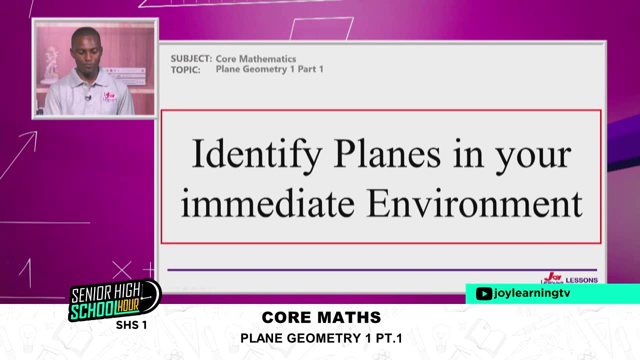 the same as that, and we can have this also going this way, and we can have this going that way and we get three dimension. and so for what we are going to look at today is two dimensional figures. so we identify planes in our immediate environment by the definition that we have here if we say plane. 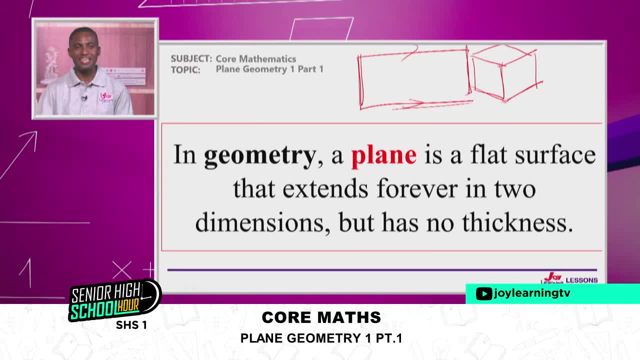 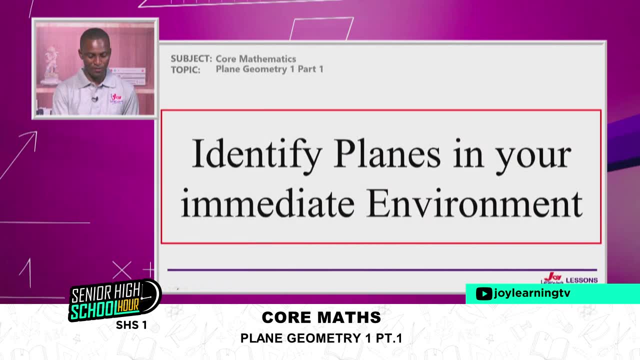 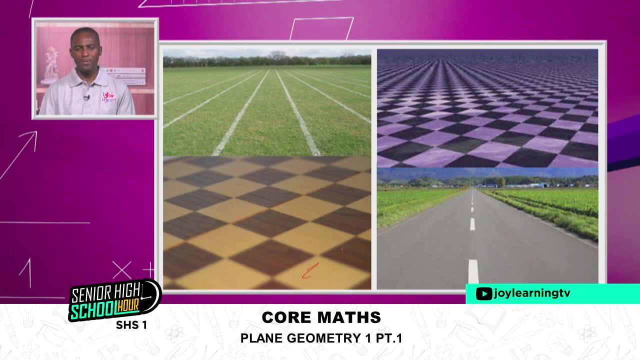 is um a flat surface that extends forever in two dimensions and has no thickness. how do we identify things around our environment as planes? so you can look at a field here, you can look at this um a room, carpet or something i mean. plane is a flat surface, it's infinitely long and um it's, i mean extend. 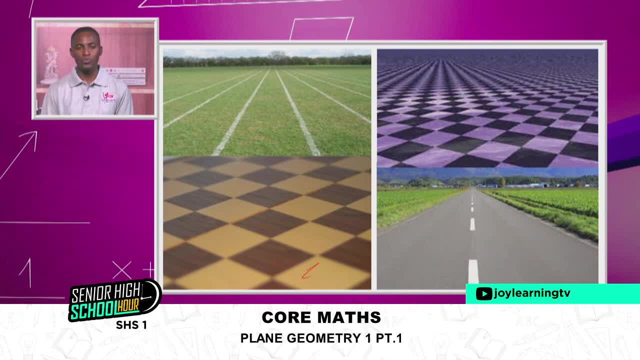 forever and there's no thickness. so indirectly, what we are saying is that we can't hold plane plain figure. you can't hold plane figure, you can't hold it. and so sometimes you tell us that you can't really say, oh, but you can hold a paper like this one. 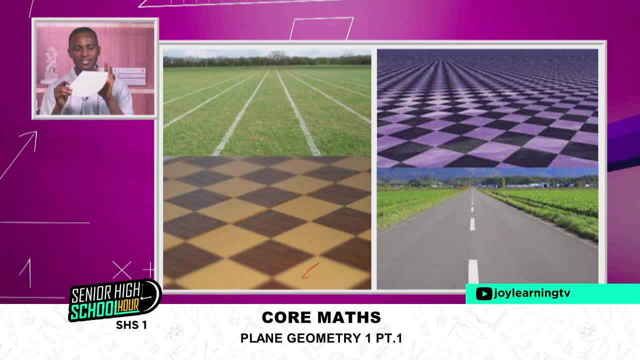 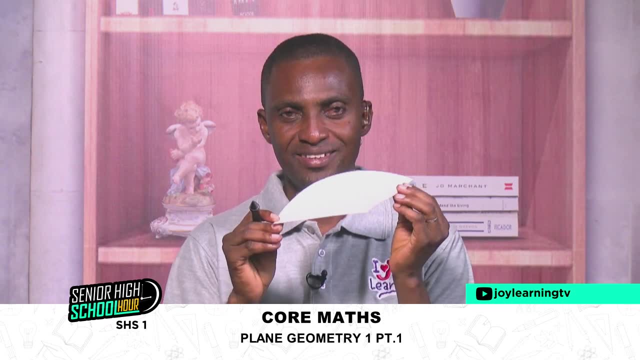 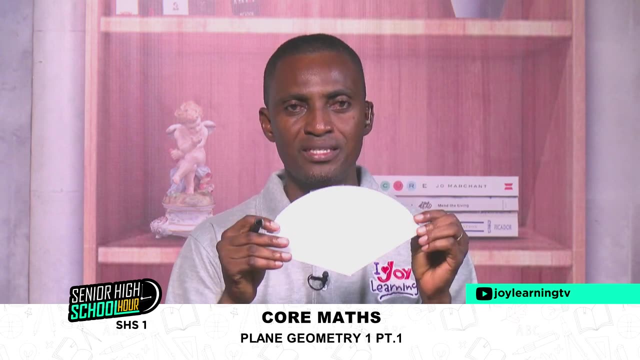 yes, paper. this paper has a, a shape, and this is um um, sector, right, but i can hold it because it has a thickness, okay, but if there's no thickness, then the surface we see here becomes a plane, some surface, and this plane shape is a sector, right. so that is what plane is all about. 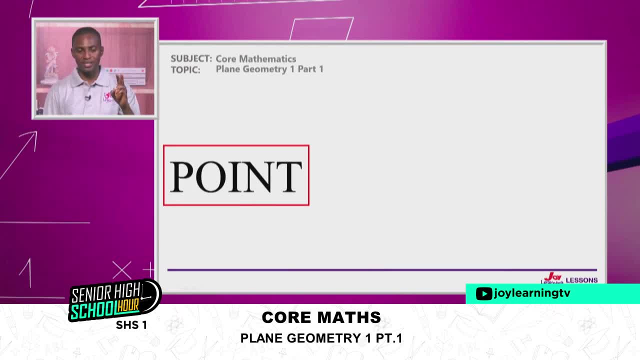 then let's talk about point. remember, we are talking about three undefined terms. i've mentioned the plane, the second one is point, then the third one is going to be the line: what is the point? what is the point? what is a point? normally, if you ask this question in class, students will say: point is. 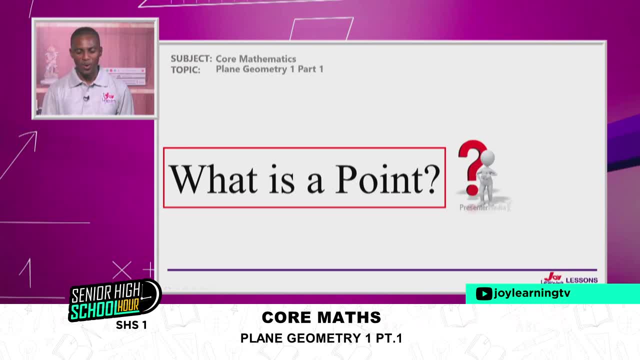 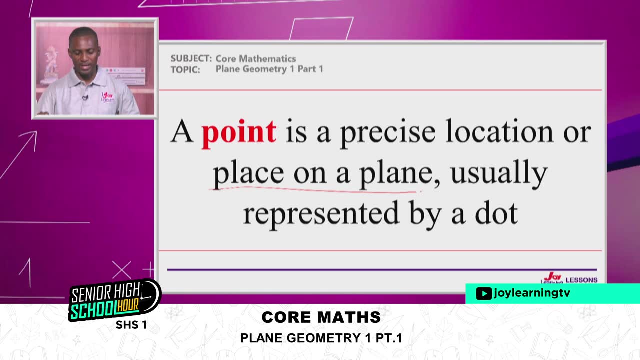 a dot. no, point is not a dot. okay, point is a location. is a precise location or a place on a plane. usually we're represented by a dot. it doesn't mean dot is a point. you, you use dot to represent a point on a plane, but ideally plane is a location. 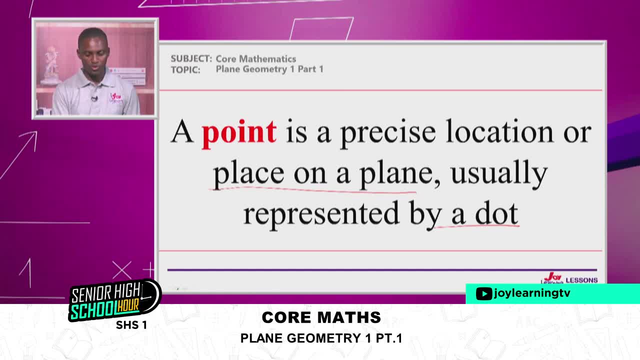 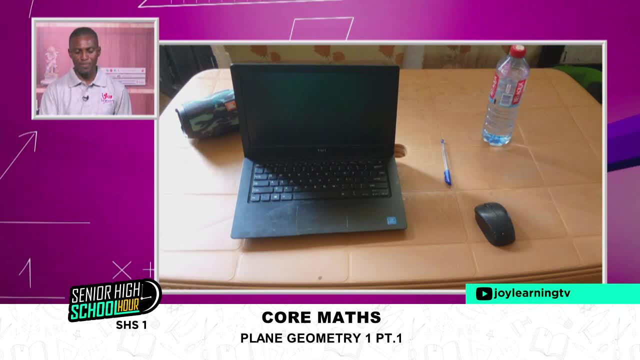 or a place on a plane. so if you look at this example here, you see a table which is a plane, and i have a laptop here, i have a pen, i have a bottle of water, i have a mouse, i have a speaker. they are all on top of this table. so if the table is, 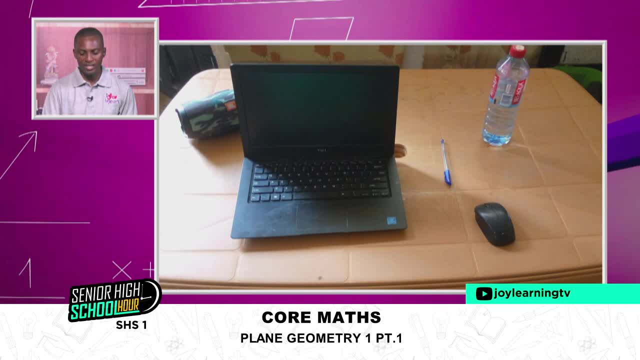 a plane, then the position of each of this object is the location, that is the point of reference. and so, on this table, the mouse is at a particular place, so that is the point. the laptop is on a place, or it's at a place, the water is at a place, so the location of. 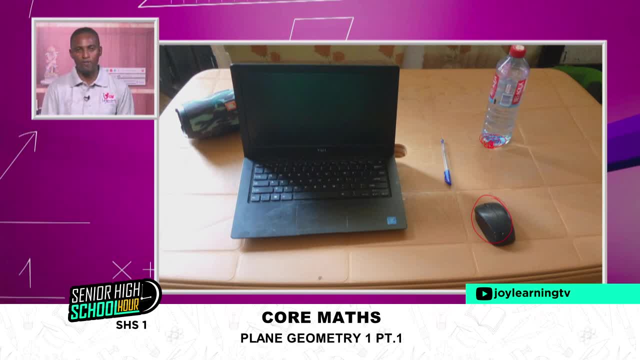 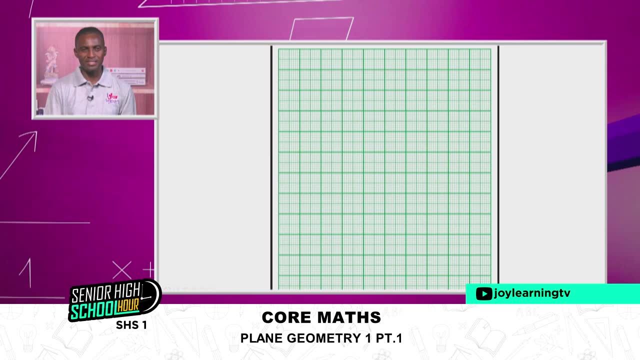 the water, i can put a dot there to show that that is the point of where the water is located, right? so that is that when you come to mathematics, normally when we are talking about points, we normally represent point on a cartesian plane. so if i have x and y axis here and i locate 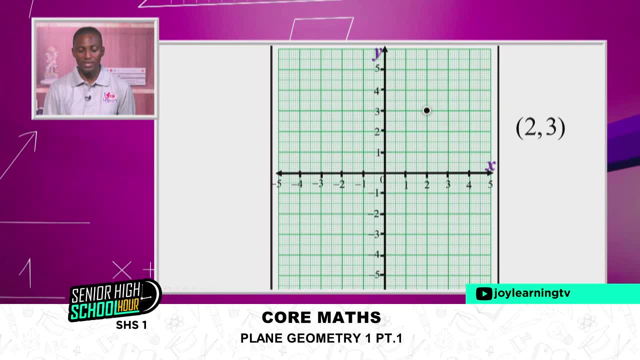 um, a point which is, let's say, point a. let me call point a, and the point a is a place. it means, if i start from the origin here, for me to locate that place i must move two steps on the x-axis and three steps on the y-axis and i'll get to the place. and so if this place is an origin where you 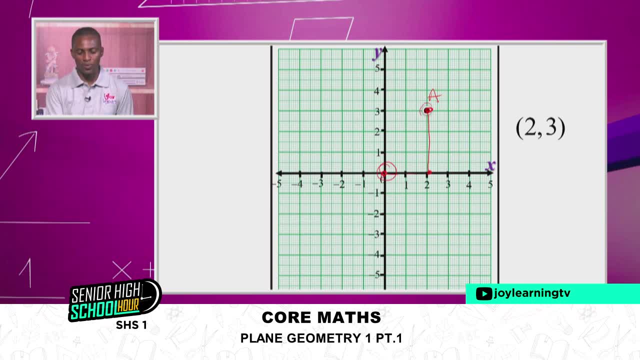 are standing right now and you are asked to locate a town called town a, and then the dimension giving you is that move two steps on the x-axis and move three on the y-axis. you locate a place called a point. point a is a place on this cartesian plane, right? 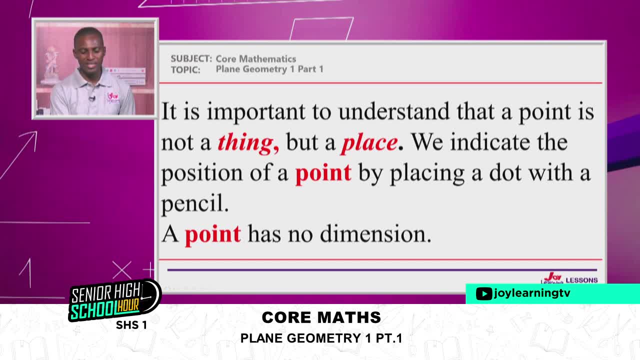 let's take note of this. it is important to understand that a point is not a thing, but a place. like i said, we indicate position of a point by placing a dot with a pencil or any other thing. a point has no dimension. take note of that. it has no dimension because it's not a thing, just a place. 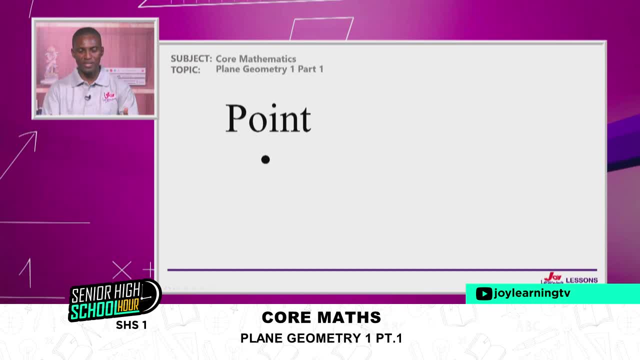 so i can locate point with dots. so you can see this plane here. i can locate the dot. i can also locate a point on a line. i can locate a point on a line. let's assume that, um, this point are places in a particular place. okay, and if they are on the same straight line, then it. 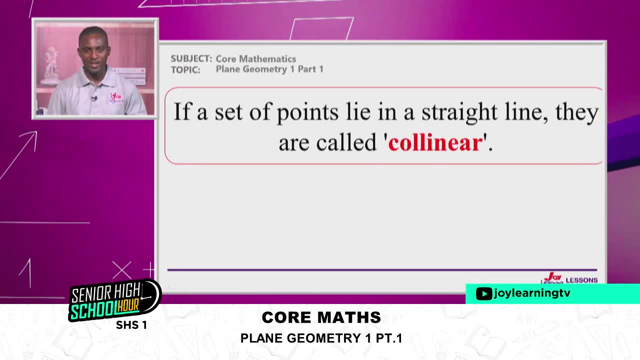 creates what we call colinia point and so we have another term we call colinia point, which means if i set of points lie in a straight line, they are called collinear point. so if i have countries and all the countries on the map can be located on the same straight line with dots, then we can. 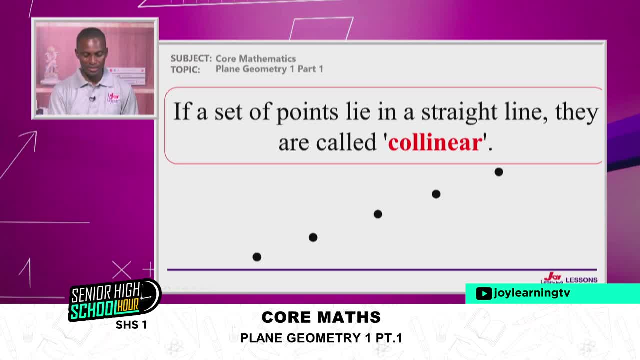 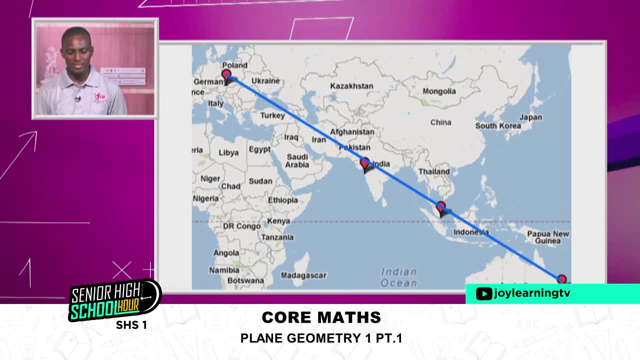 see, those countries are collinear countries. that means they are on the same straight line. so points that lies on the same straight line are called collinear point. and so if you look at this map, look at the country that um, germany. we have in india. here we have um maybe indonesia, australia. 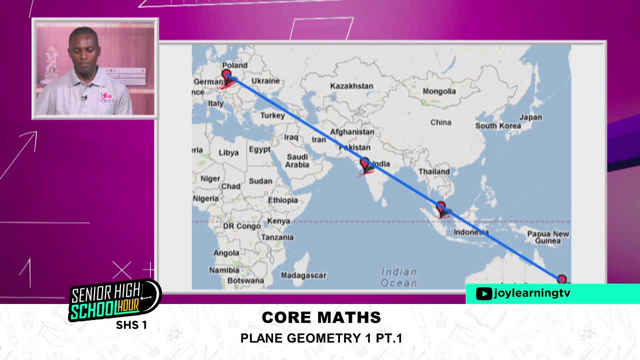 you can see that if you track these countries on the map and you draw a line through all the places that they are located, you see they'll be on the straight line. and when they're on the straight line we say they are in collinear. i mean the points over there are collinear points. so the 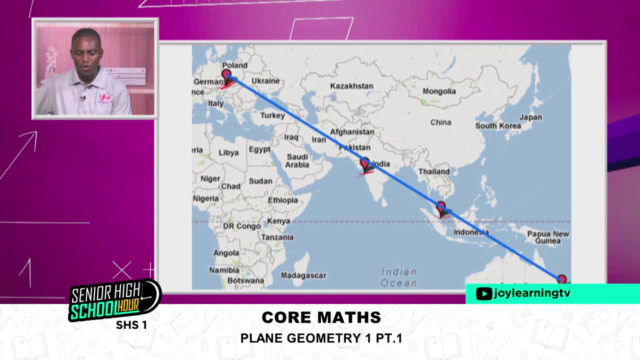 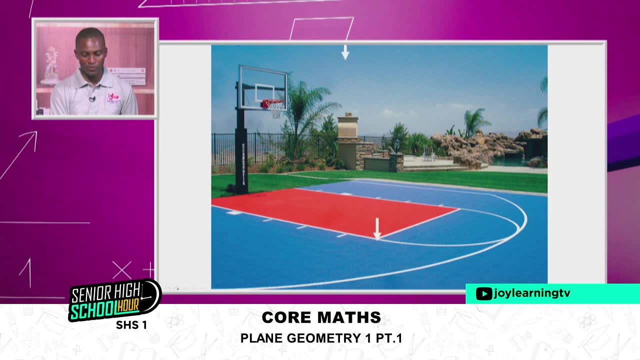 countries can be called collinear countries. that means they lie on the same straight line on our map. if you look at this particular field too, you can see the location of this, location of that. they all are on the same straight line, and so we can say they are collinear point, collinear point. 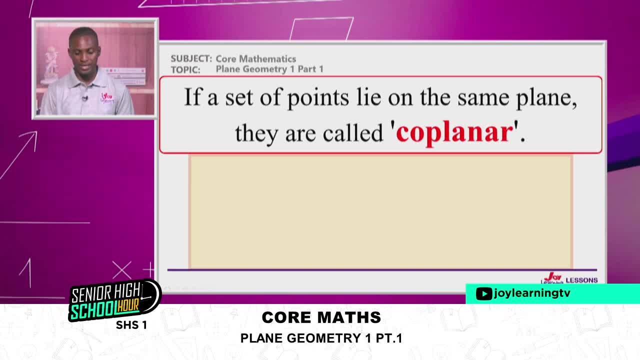 then again, if a set of points lie on the same plane, they are called co-planner, and so let's have this our a plane, and i locate point a here, point b, point c, point d, point e. you see that they are not necessarily on the straight line, but they are all on the plane, and so we see their co-planner. 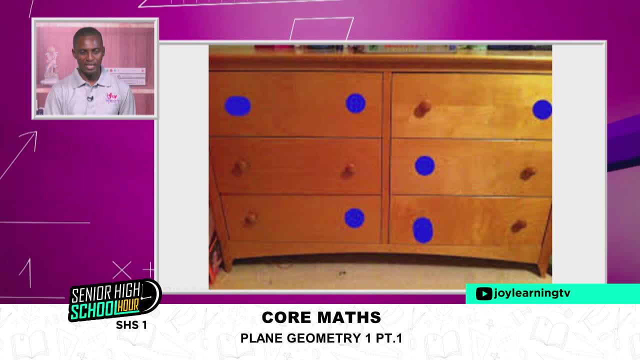 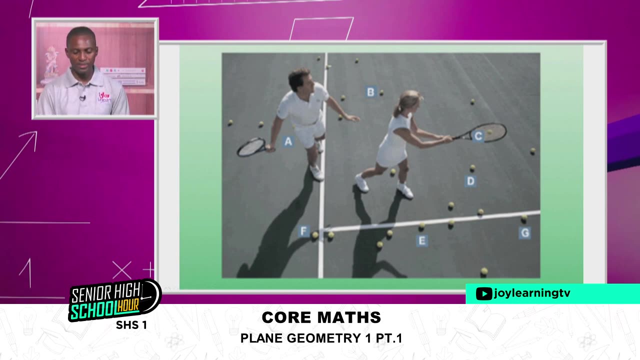 i see their co-planner, so you can see that on this sideboard here you can see this, um spot of the blue. i mean that makes a co-planner on the same plane. and if you look at this picture, here too we have um tennis balls. they are all on the flat surface. 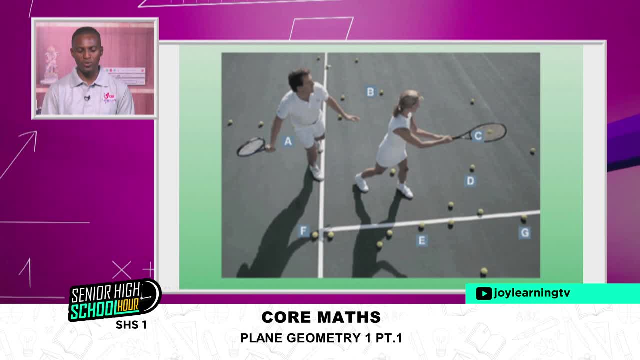 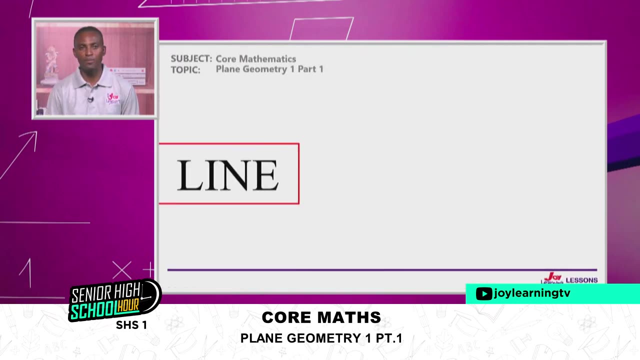 and you can see here that um, those tennis balls can be considered as co-plan. i mean they are located on on on the um field and so they are co-planner. the position of the balls are coplanar because they are not on a straight line. then the last um, undefined term. we want to talk about that. 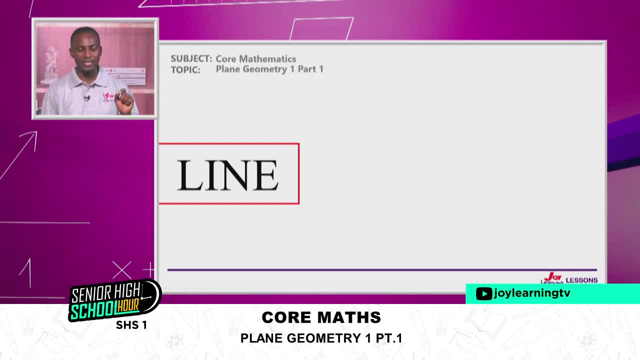 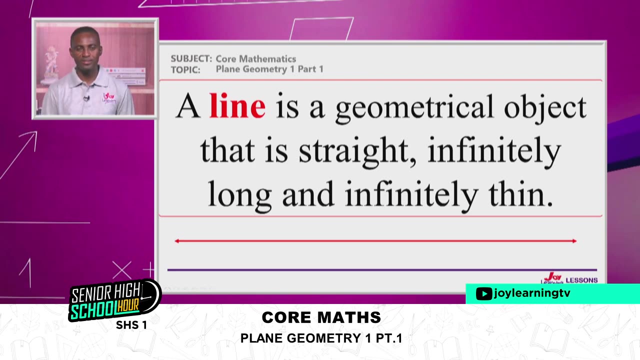 will help us to define all other geometrical terms. is line. what is a line? what is a line? that's a big question. i want to ask: what is a line? in geometry there are a lot of definitions for line, but then in geometry we can consider this: 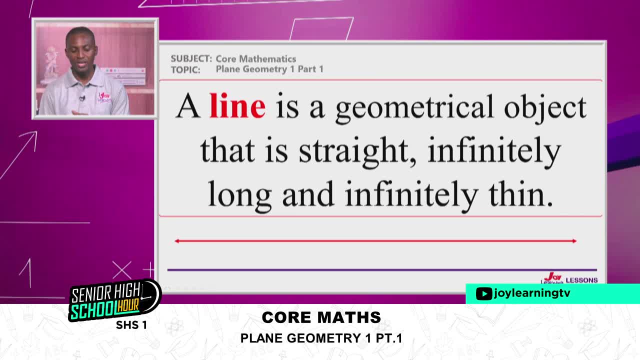 definition as um. a line is a geometrical object, because we are talking about geometry. it's a geometrical object that is straight, infinitely long and infinitely thin. that's a line. so ideally we can't draw a line because it has no beginning, it has no end, it's infinitely long. so if you want to draw a line, i mean you can't. 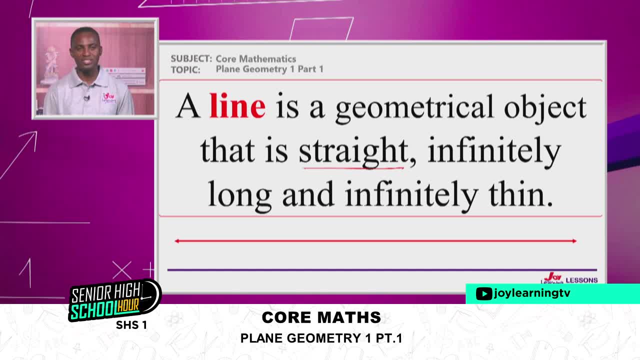 finish drawing it. that is why, in drawing a line, we use this arrow to show that it has no beginning, it has no end. so what you see here is a line, because i've indicated with an arrow telling you that there's no beginning and there's no end. and so anytime you draw a line and you want us to know, 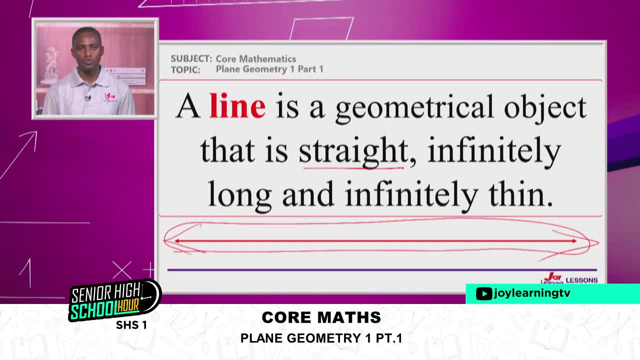 that that is a line you must indicate with arrows to show that a line. i don't like to be something different. that is why in drawing normal line you always see that we draw number line and we show these symbols and then we indicate our maybe zero, and then one, two and three, and we go that way even. 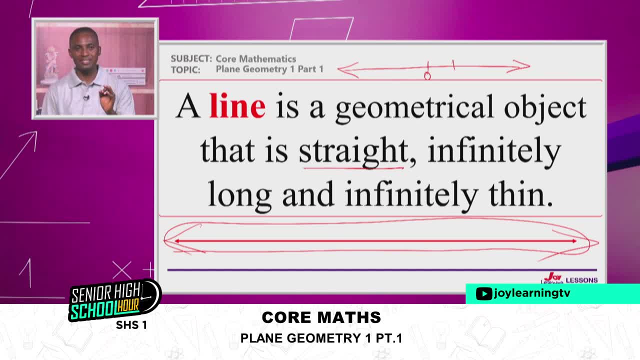 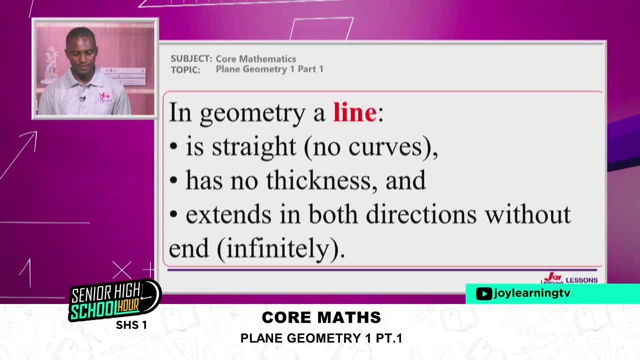 in cartesian plane two we show with arrows to show that the x-axis is a line, so it has no beginning, it has no end. and so in geometry we are saying that a line is straight. that means no curves, it has thickness, so it has no thickness, sorry, for that has no thickness and it extends in both. 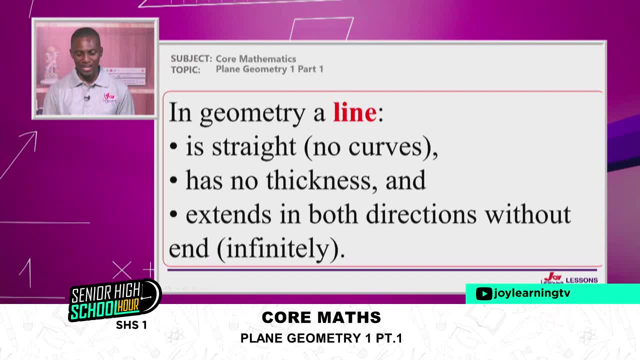 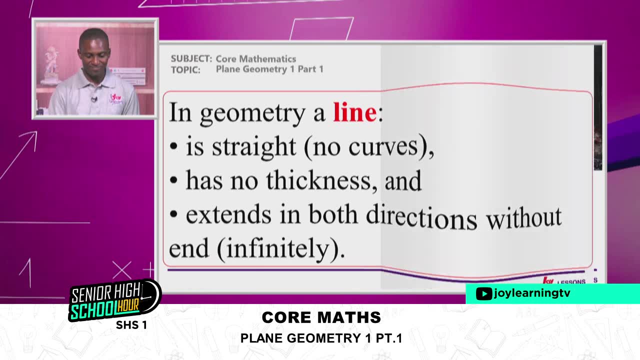 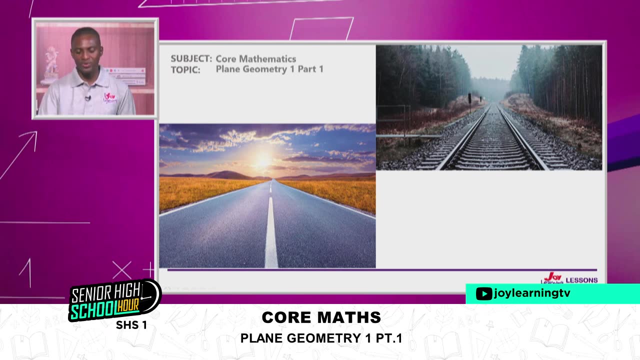 directions without end. so we say it is infinitely long, right, so i can have a railway line where we see that the railway has two lines and it has no end. so we say it is infinitely long, right, no beginning, there's no end. it goes on and on, even though there may be a beginning somewhere. 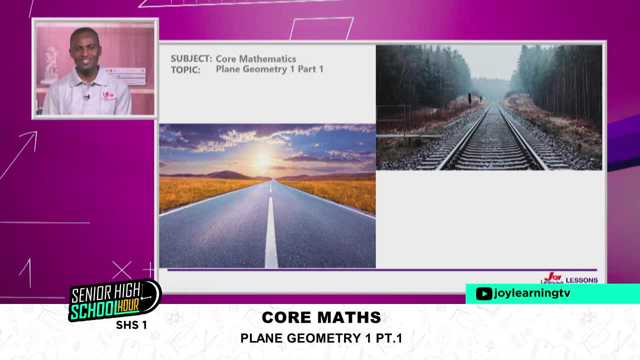 but at any point that, where you see it, you see that you can't track the beginning, you can't track the end. or let's probably go to the railway station where you see where it starts, then you can think of that. but when you meet it in town, it's like there's no beginning, there's no end, because 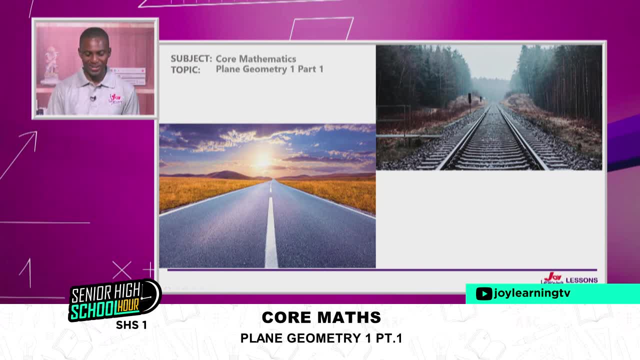 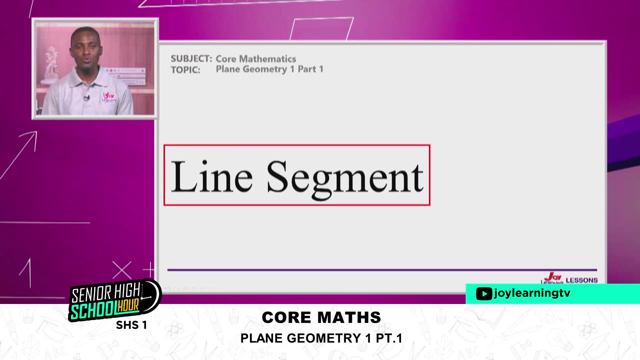 you keep following it. you work and work and you get tired and you have to stop right and if you see a rose to almost the same, sometimes you want to track a road. you continue when you realize you right. okay, so that can represent um a line. then we also talk about line segments, and this is what 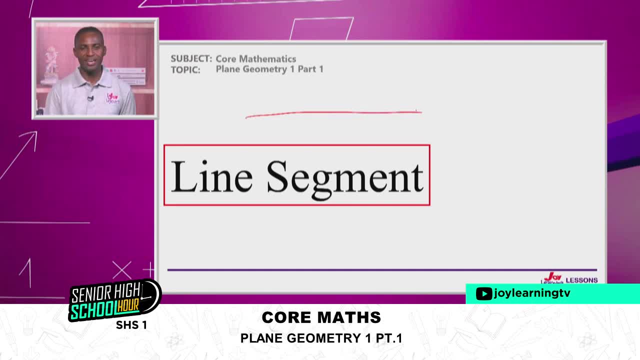 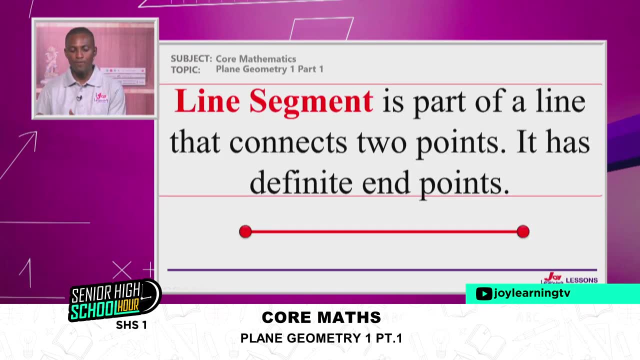 we draw almost every now and then they want to draw a straight line. then it means, um, you've drawn a line segment and we are saying, by definition, line segment is part of a line that connect two points. it's part of a line that connect two points. it has definite end points. 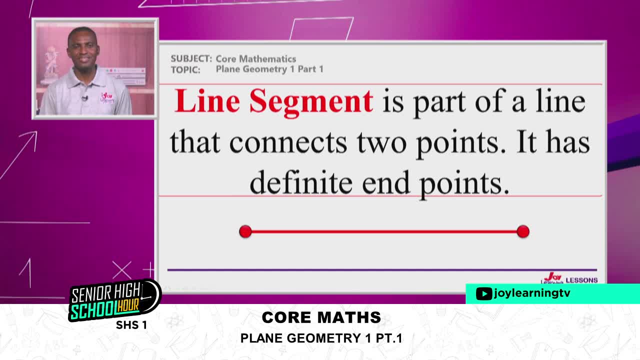 in some cases we see people defining line as a line is anything that exists between two point. when you define a line by saying it exists between two points, then you are. you are talking about line segment, but not line. line has no beginning, it has no end, but line segment has a beginning and it has an end. so 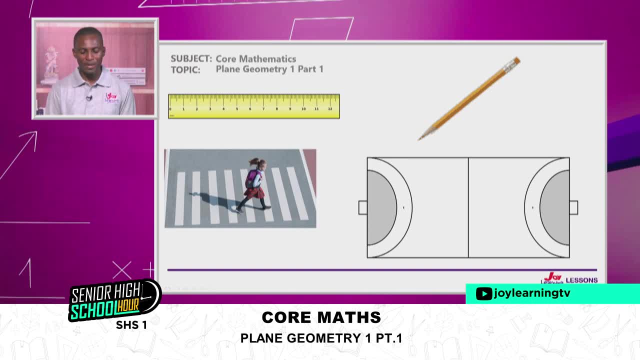 that is lying segment for you. and you can see here that if i pick my ruler and i have a beginning of the ruler here, the end of it here it can be a line segment. the pencil has a beginning, it has an end. we create a line segment for that, even on our fields. um, let's say you have a basketball field and other. 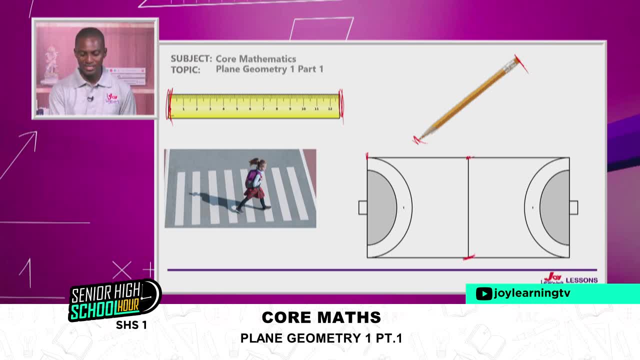 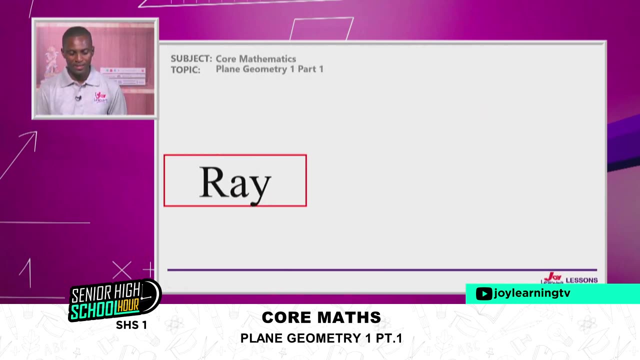 stuff. you also see line segment. so this one starts here, it ends here, and then on our rows we see this max that is used to indicate zebra crossing. they are all line segments, they have a beginning and they have an end. very interesting cause. right, that is um geometry for you. it's a very wonderful. 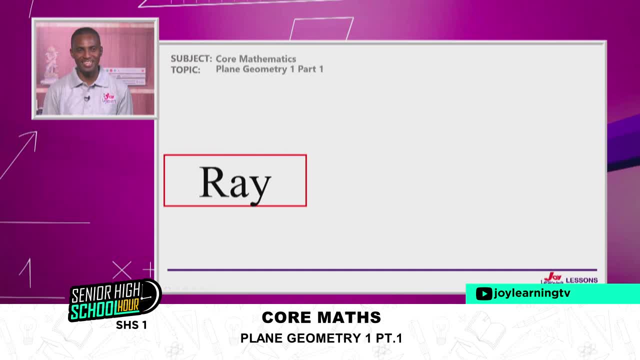 because geometry is all around us. we see it every day, in fact. without geometry, um, the world would have been a bit weird. i mean, we wouldn't see the beauty of the world because geometry is giving us that sort of beauty that i mean angles and the shapes and stuff. let's talk about ray ray, another. 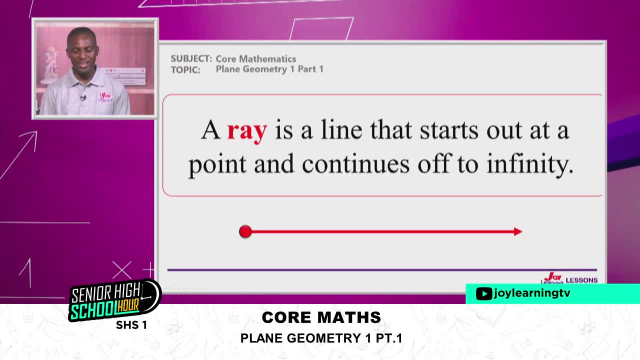 line we want to talk about is ray. a ray is a line that starts out at a point and continues off to infinity, so it has a beginning but no end. in fact, this reminds me of a man in the bible. the bible says, um, he has no beginning, he has no end, and i'm sure you know that person, mckinsey. 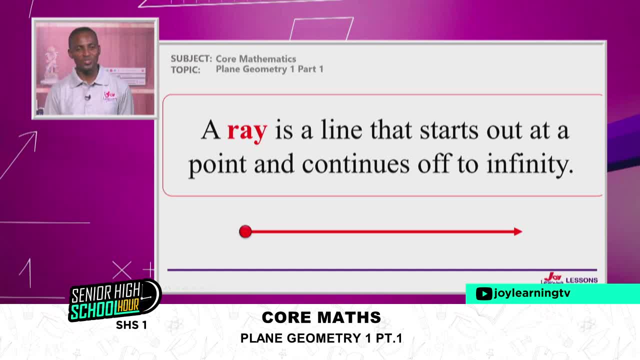 so mckinsey can be like um a line. he has no beginning, he has no end. that means there's no um a point where we can make a reference that he was born on this particular day and he died on this particular day. he was not born, he didn't die. so it's like a line. 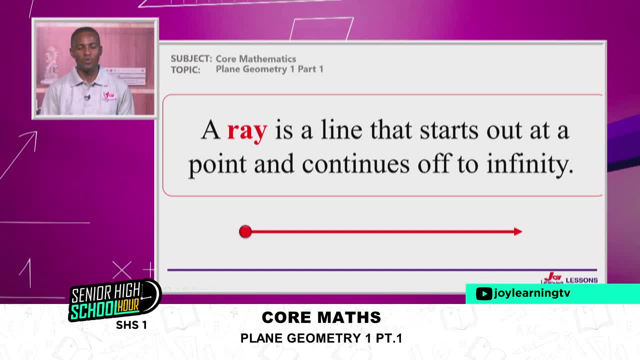 that we have those of us who were born and then one day we die. i mean we will represent the line segment right, because you have a beginning, we have an end and we have others too who had beginning but they didn't have an end. i mean they didn't die, they live forever, and example is um. 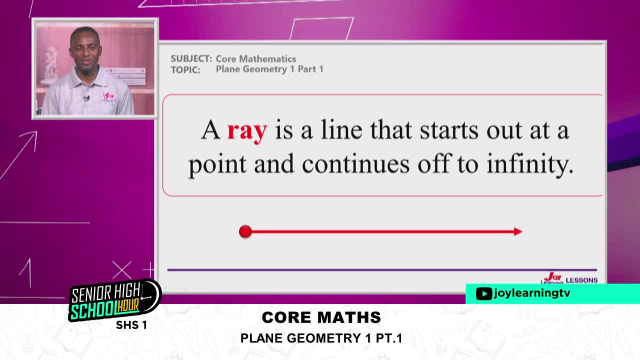 enoch. enoch was born, but he didn't die, according to the bible. and um elijah was born, he didn't die. so it's like a line segment and mckinsey will be a ray, whereas maybe anybody who was born and died will be a line segment and mckinsey will be the um, the line who has no beginning and has no end. now, 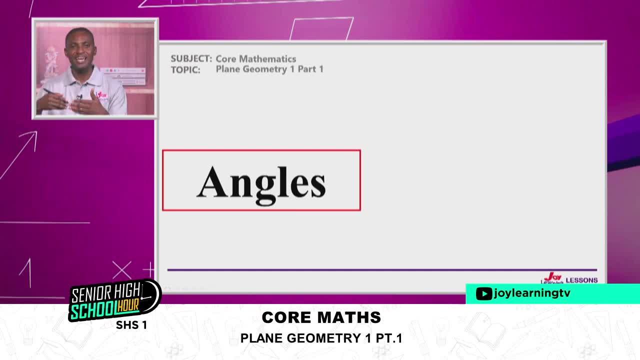 let's talk about angles. now we've been able to talk about the undefined terms: the line, the point and then the plane. now, based on this theory, we can define all other geometrical figures. so example of geometrical figure is an angle. so let's talk about angles. 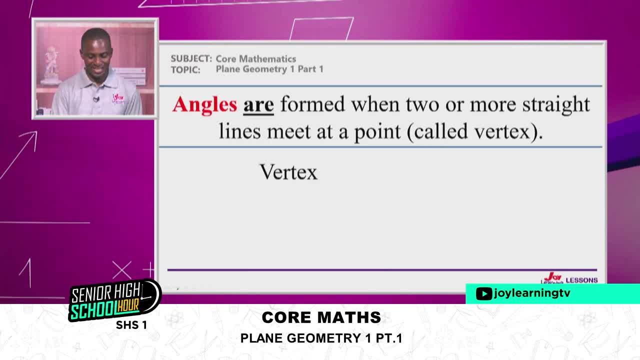 what is an angle? what is it? what is an angle? angles are formed, and i'm underlying the word are formed, because some cases people will say: angle is formed. then when you draw two or more straight lines, you create angles, and so angles are formed when two or more straight lines 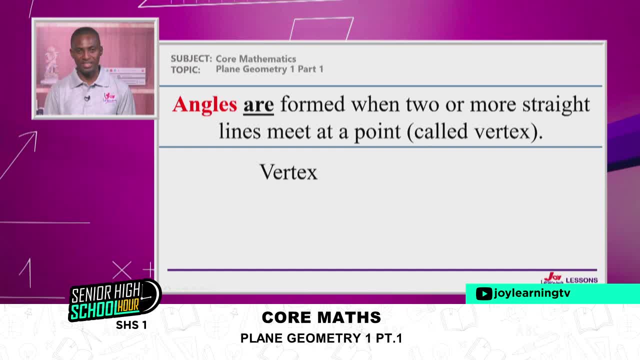 meet at the point and the point they meet is called vectors. okay, so that's one definition. but when you search for definition for angles, you have about thousands of them. they all point to one formation. i mean one thing. that is what we have here. so if i have two lines meeting at a point and the point is called vectors, 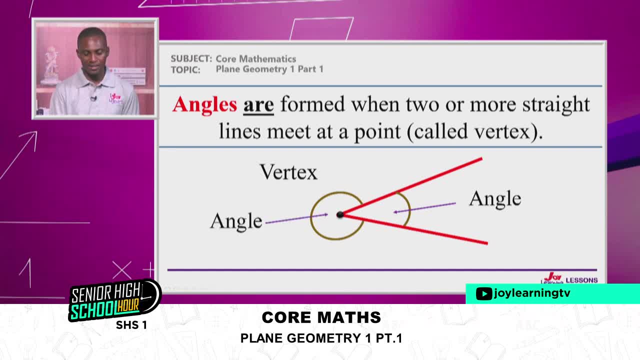 then we create two angles here, so you see where the angle one is and then the other angle is. so let me call this angle one and angle two. in future we're going to learn to know that angle one is reflex angle and angle two is an acute angle because it's less than 90.. so angles are formed. 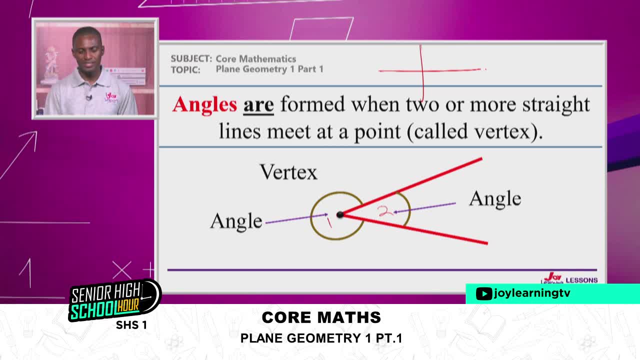 when two lines meet. so even if i draw this, two lines meet here- we have four angles created here. can you see that if i do this, i have four angles created, and so angles are formed when two lines meet at a point. then we have this one called the arm of the angle or the side, some cases. 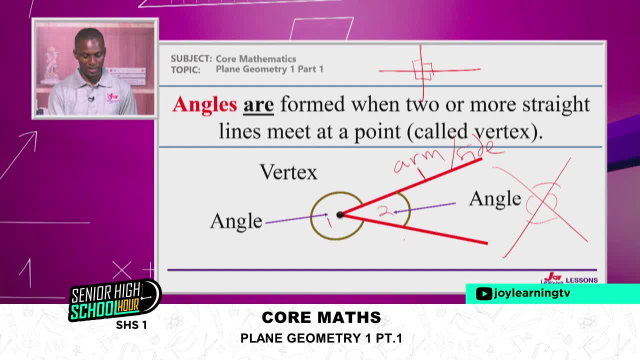 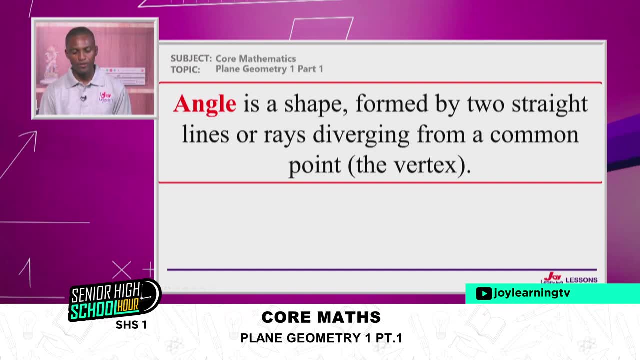 we call the side of the angle. okay, so the arm or the side of the angle. then others will define it as this angle is a shape formed by two straight lines or rays diverging from a common point. so you see, they diverge from a common point. so two rays diverge from a common point. we create angles over there as well. once. 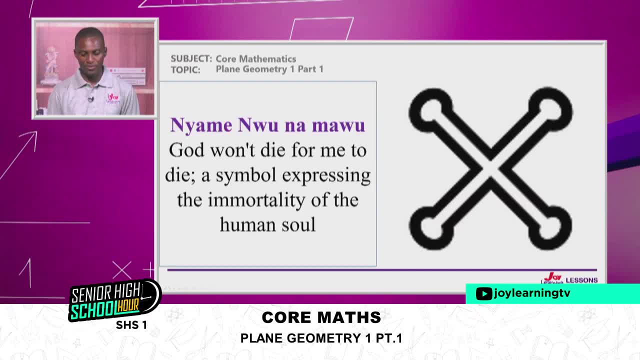 again, we have our vectors at the meeting point and then we have that, and so we have angles everywhere. this is a drinker symbol. okay, and this is a drinker symbol we can see angle created here. it means we knew angle right from day one, our forefather. 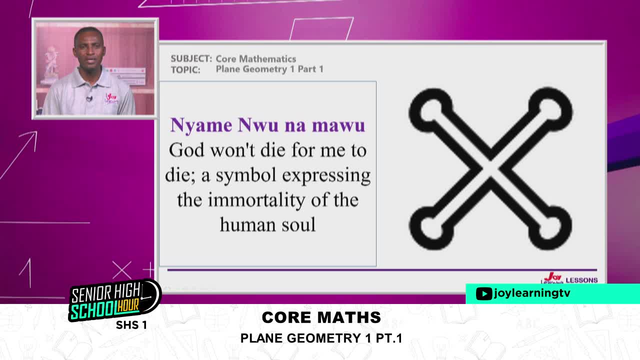 who gave us these designs new angle when they were giving us a drinker symbols. and it's so amazing that the christ symbol speaks a lot to us each and every day as we meet them in our clothes, in our walls, in books, etc. now this symbol simply says: 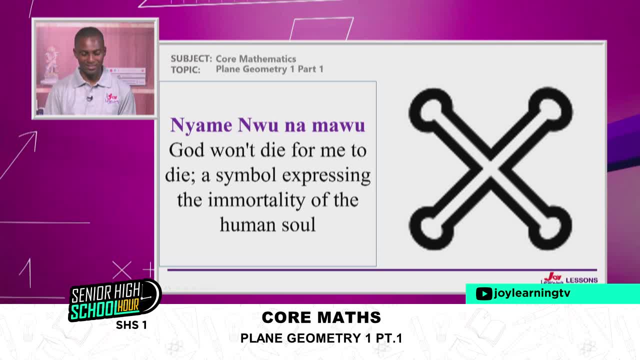 god won't die. for me to die, a symbol expressing the immortality of human soul. it means that if we die as far as god remains, god will not die. our soul will stay forever. so, even if we die today, our soul will never die, will remain to eternity. that is why you have to give your life to christ. 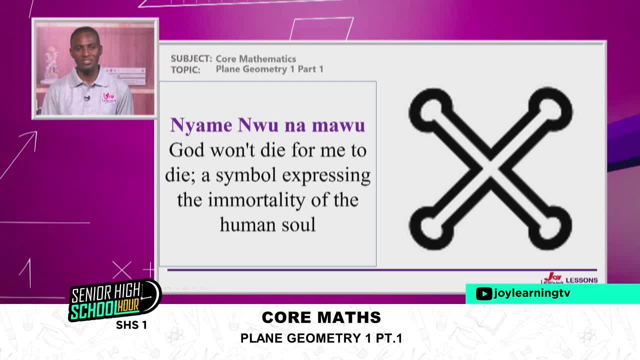 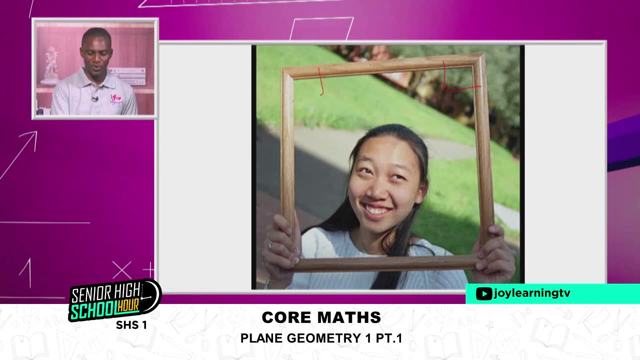 so that when you die, you know you can stay with god forever. if not, then whatever happens, the choice is yours. all right, so that is, we can see angles here. as we look at this aging symbol- in fact, a lot of them has a lot of angles- and then you look at this object, you can see an angle everywhere, i mean. 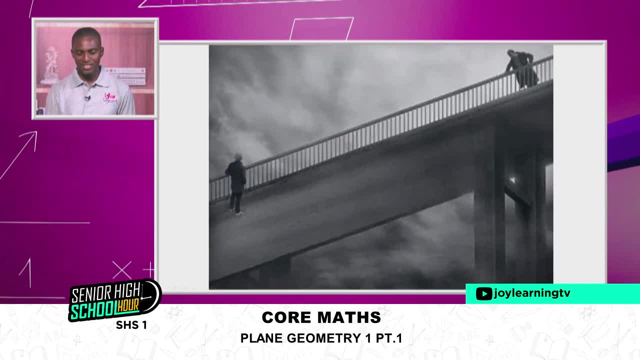 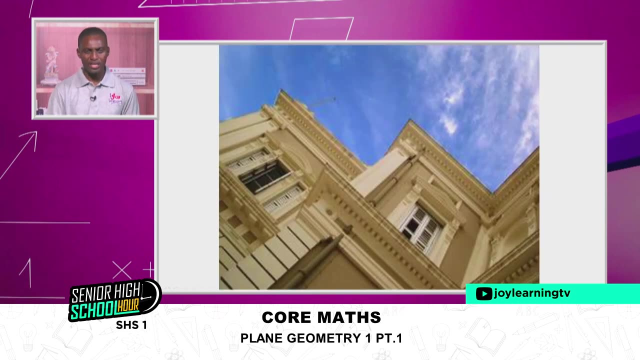 angle everywhere. you can see the bridge here. angles are located every aspect. so we see that in our everyday life. we design buildings, we build other artifacts, and angles is everywhere, even in our buildings. we see angles in our windows. i mean even the food that we eat, some of the food we have angles in them. oh yeah, that is true. 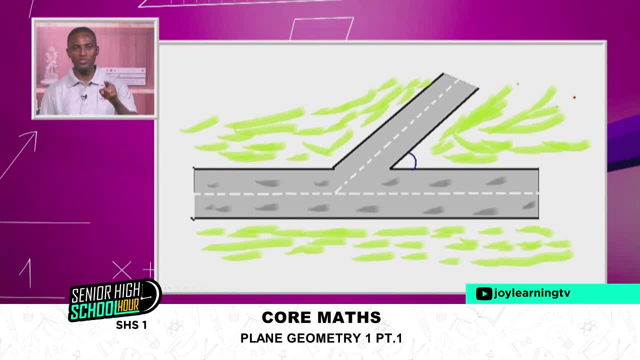 on our roads. we see angles and they'll tell you: oh, when you get to a t-junction, the teachers. you see an angle over the right, god you see, you get wide tension, and i've been hearing this every now and then. so we see angles in our everyday life. we see this plane here, an angle is created there. 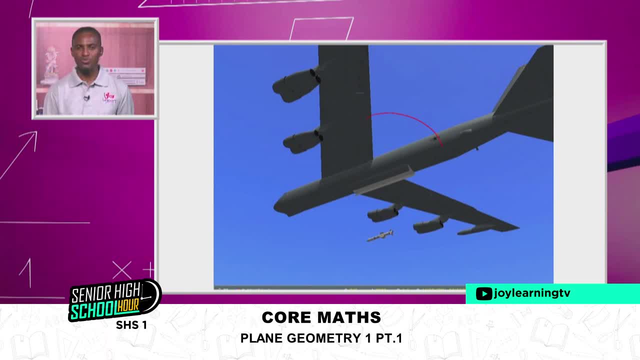 and so the designer of this plane knows about angle. that's why mass is very important. masses are everyday language, so you can't stay without mass. people ask questions. we do all this, in fact, without mathematics. you can't speak in this one and clarify things, because if you're an engineer and you want to express why you did this particular plane in this particular 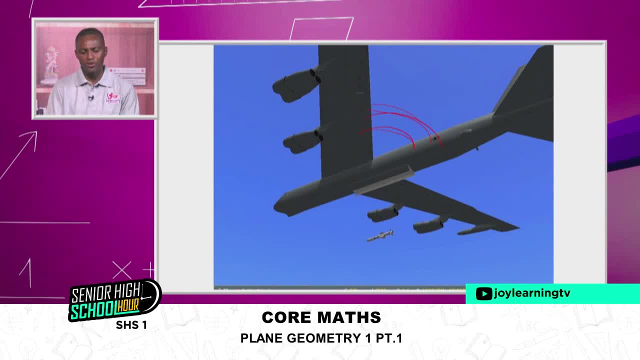 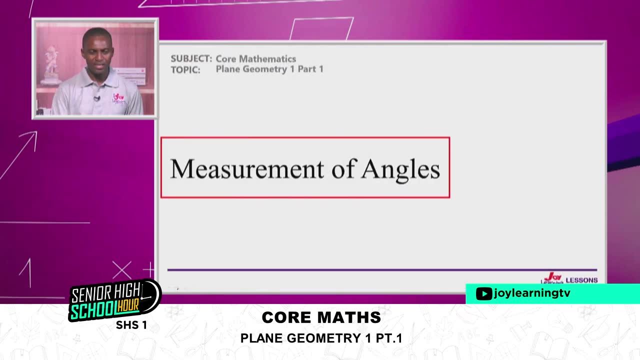 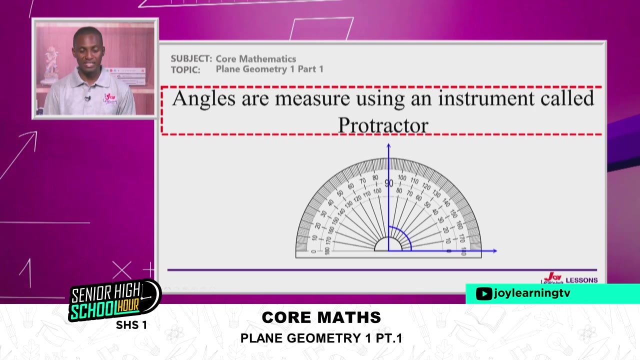 design, you should be able to use the term angle, or the angle between the body and then the the rings. is that? i mean that is um angle for you. now, how do we measure angles? how do we measure angles? angles are measured using an instrument called a protractor, and we can see it on the. 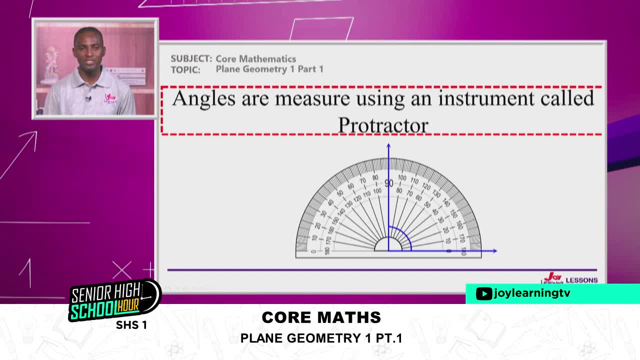 screen here. that's our protractor, and i'm sure you know how to use it in measuring angles right from primary school you were taught how to use protractor in measuring angles. they are measured in degrees, so when we're talking about angles, we're talking about 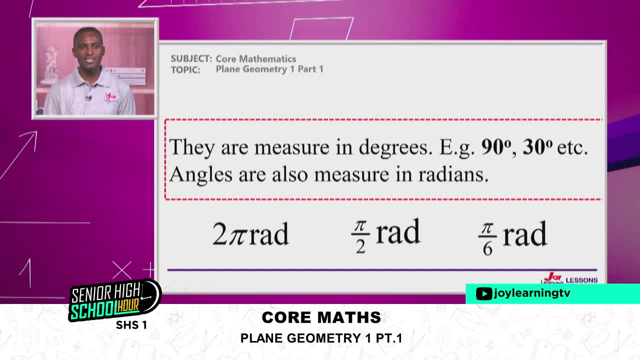 degrees, because angles are measured in degrees. in some cases, to measure angles using radians, we use radians and sometimes we use grades to measure angles. and when i do elective mass in some aspect of trigonometry, they'll ask you to leave your answers in the radian. so if you have, let's say, 180 degrees, you know that to be pi pi radian, so pi radian gives. 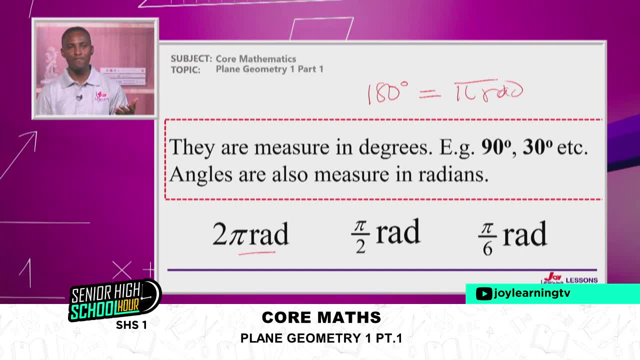 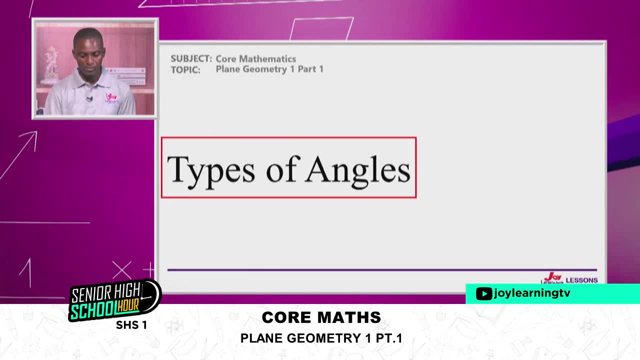 you 180 and then 90 degrees will give you half um radian, so half pi radian. i mean that's that types of angles, very important concept we need to understand because as we speak and use the language of angles, angles comes in different sizes and different shapes and we should be able to use 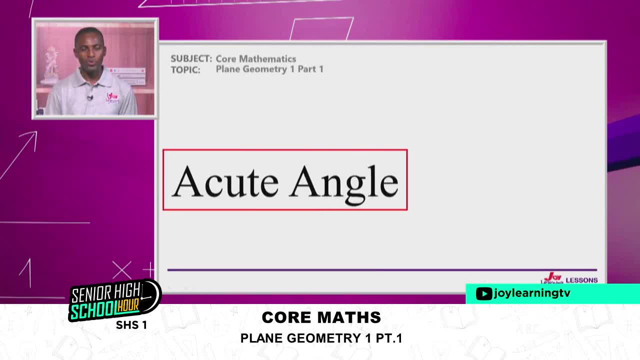 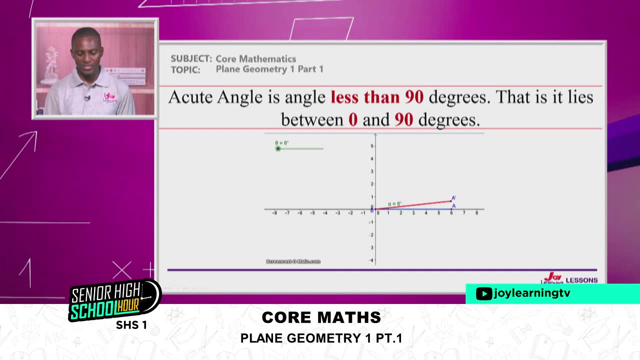 the correct language to express them. we have what you call acute angle, acute angle or acute angles by definition. here we say that acute angle is an angle less than 90 degrees. it's less than 90 degrees. so if you look at this diagram here, you see that all the angles right from zero. sorry. 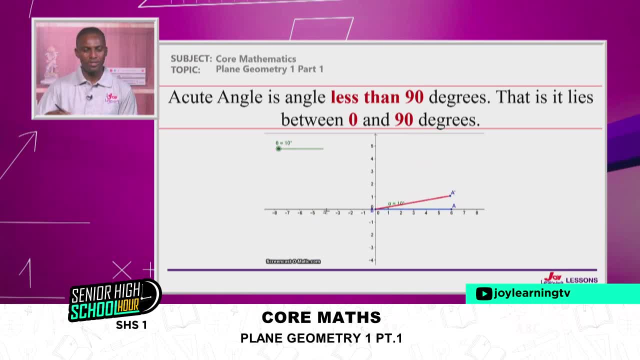 right from maybe after zero, one to three, up to 89 point, whatever those sort of values, between zero and ninety. any angle. there is called acute angle, so it lies between zero and ninety. all we can say is an angle less than 90 degrees. now i'm saying less than 90 because if you come to the zero, zero doesn't create any. 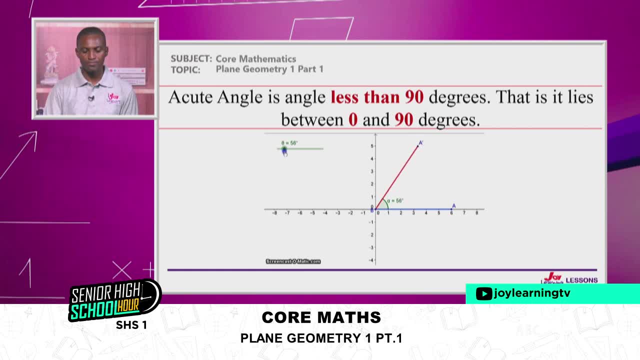 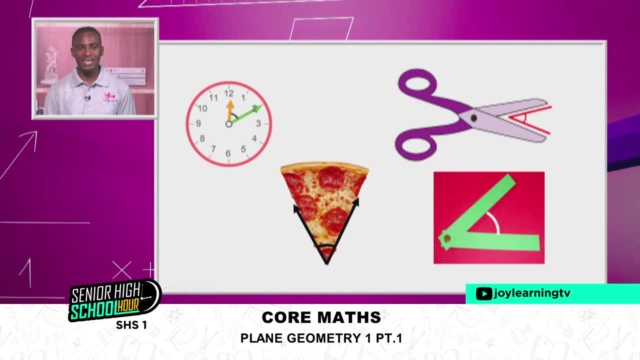 angle, so we wouldn't even talk about it, and so we have um in an angle less than 90 degrees. so in real life situation we see angles in acute form, sometimes when your time is um, let's say um 12, 10, the angle between the hour hand and that of the minute hand. 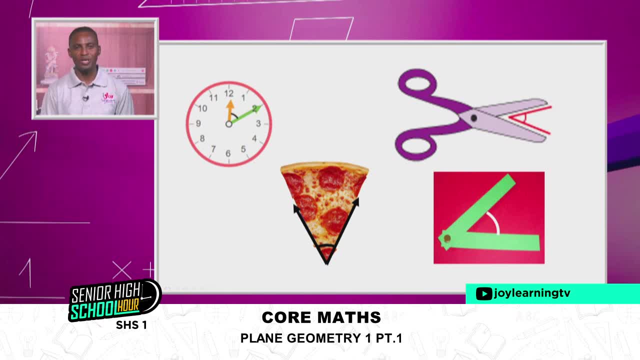 creates an acute angle when you slice your pizza, sometimes, most of times, you slice them with an angle of acute. your scissors sometimes opens with an angle of acute because this doesn't go beyond um good, your 90, but not up to more than 180, and mostly we open it to acute angle. to. 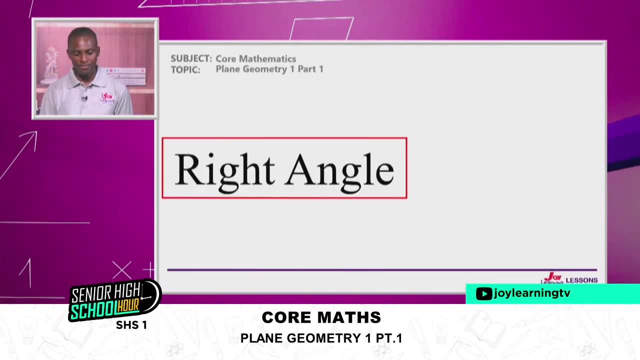 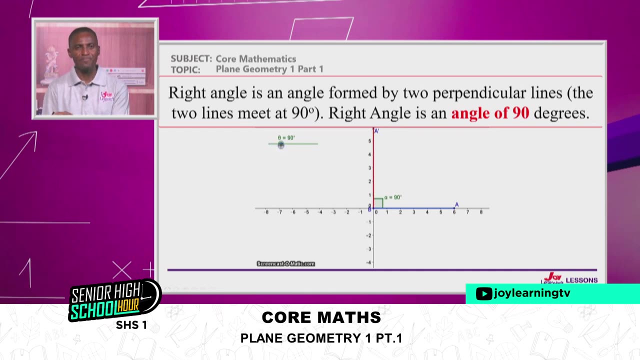 cut. so these are examples of acute angles- a lot of them, as you can see them in and around your environment. then, after acute angle, we have what you call right angle, right angle. now we say that when the angle is less than 90 it is acute. what if it's exactly 90.. it's exactly 90 then. 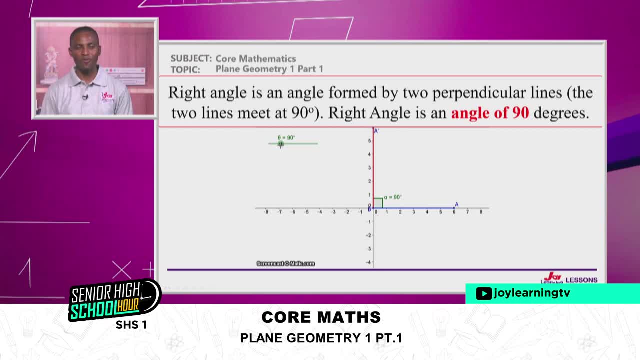 we say that what happens when the angle is less than 90 is called right angle. as i stand right now, my body and then the floor makes an angle of 90, because i am vertical and then the floor is horizontal, and so the vertical and horizontal always meet at angle of 90 degrees. so by definition, 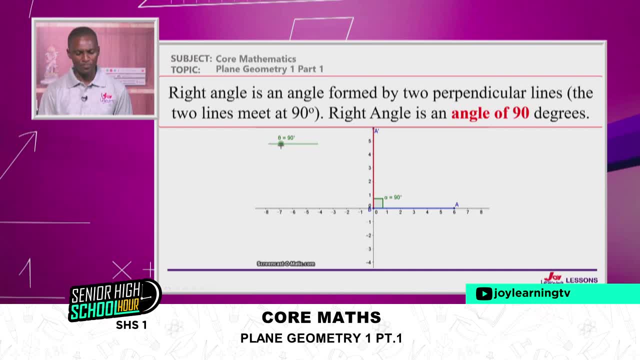 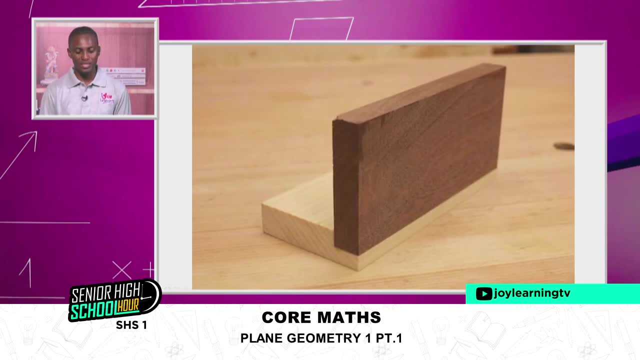 we say it's an angle formed by two perpendicular lines- we'll be talking about this in future- and all they meet at 90 degrees. right angle is an angle of 90 degrees. An example can be this: You see this particular wooden structure here. You see vertical, then you see horizontal, and that is 90.. 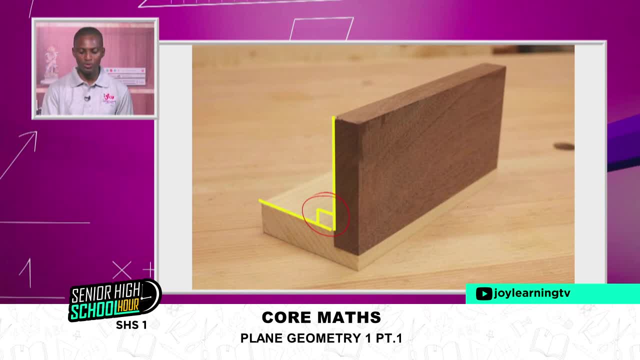 And this is a symbol we use to represent 90 degrees. So anytime you draw a diagram, let's say a triangle, and you see this symbol here, it means we are dealing with 90 degrees, or those two lines are perpendicular to each other. 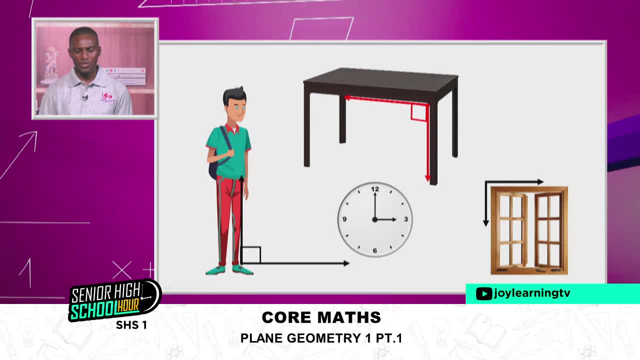 Another example: you can see when it's 3 o'clock exactly with your hour and then your minute hand. you see 90 degrees there, Your table. normally when the legs are vertical and the top is horizontal, we create an angle of 90.. 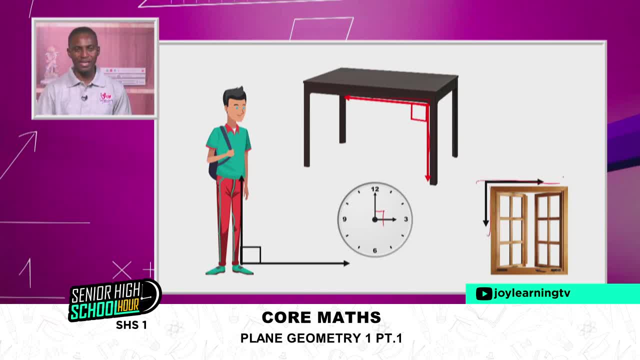 On top of our windows we have 90 degrees. When we stand, we make an angle of 90 with the floor or the ground that we are on. I mean, these are all examples of right angles. Now let's talk about obtuse angles. 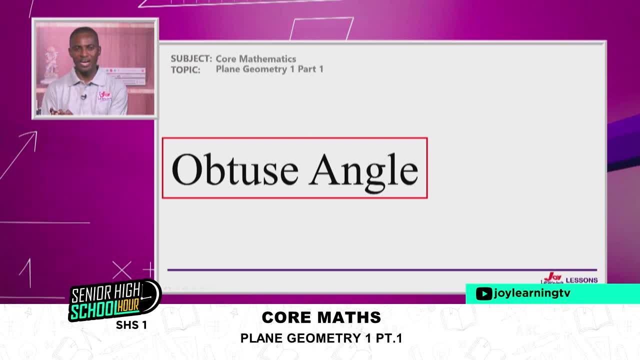 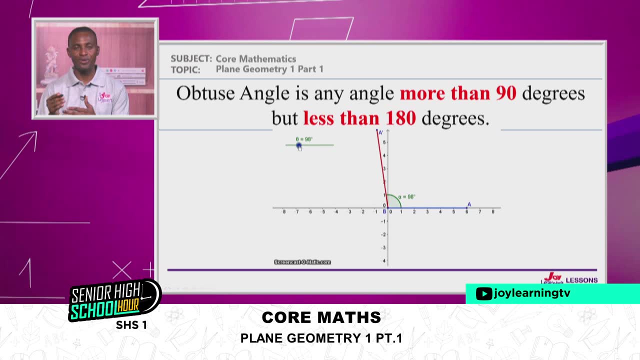 So now we are traveling Right from zero. we're talking about acute angle and we hit 90 degrees. then we change the name and we call it right angle. Now, as we travel beyond 90, now we've entered into numbers that are bigger than 90, like 120,, 152,, 179. 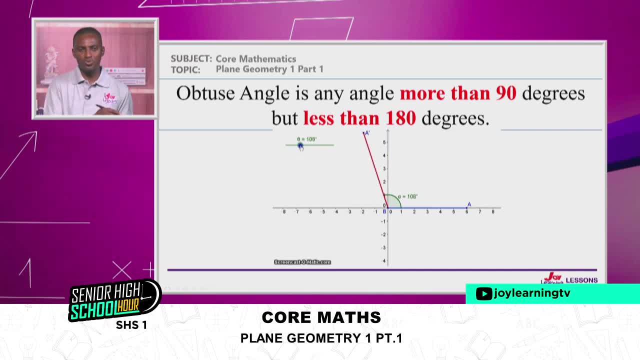 They are all more than 90. But we are traveling at 90 degrees. We are traveling at 90 degrees. We've not gotten to 180 yet. So angles that lie between 90 and 180 between are referred to as obtuse angles. 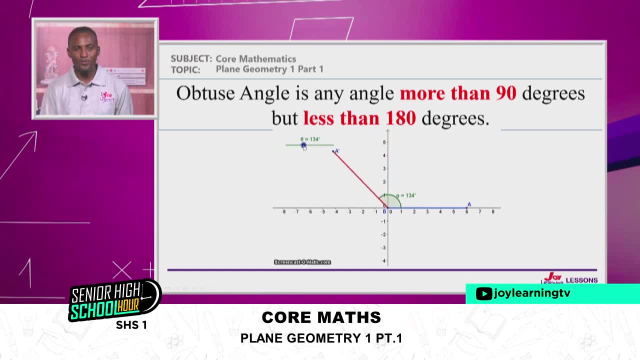 So an example of obtuse angle can be 120 degrees, 150 degrees, 93 degrees, 90.2 degrees is obtuse right. So in structures we see obtuse angle. Right now we have 90 degrees. 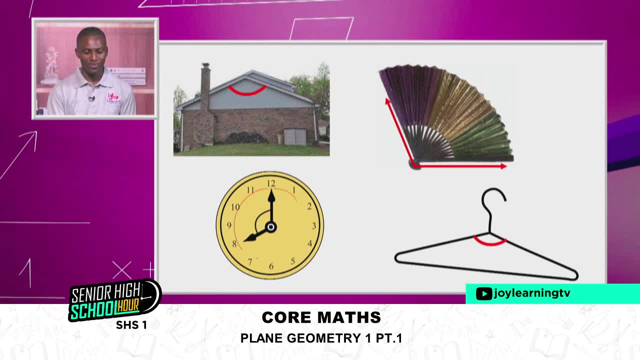 Now our time is 8 o'clock, And when the time is 8 o'clock, between the hour hand and then the minute hand, we see an angle which is more than 90.. It will be 90 when it comes, like this right. 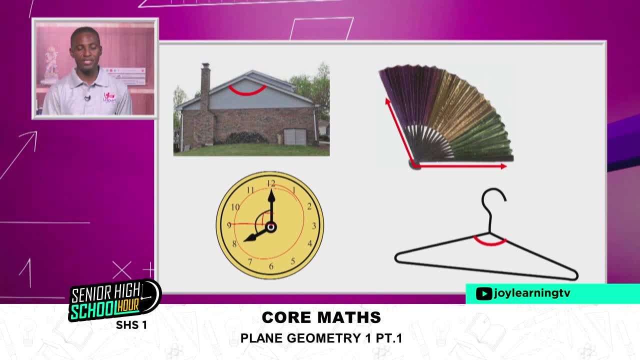 That is, let's say, if it is 9 o'clock it will be 90. But then if it is 8 o'clock it will be obtuse angle. Then on the roof here we can see obtuse angle there. 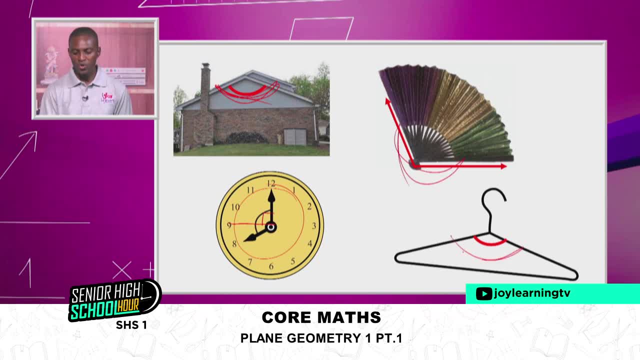 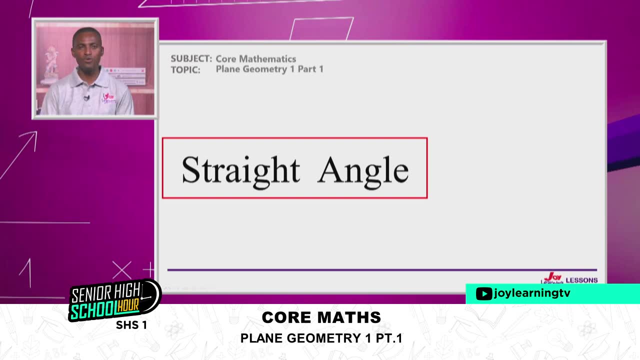 Look at this fan. here We see obtuse angle. With this angle we can. We can also see obtuse angle. So angles are everywhere, Everywhere. Then we have what you call straight angle. Now, right from zero, we enter into acute angles. 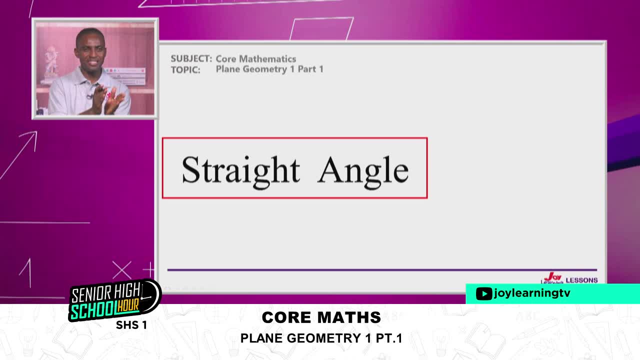 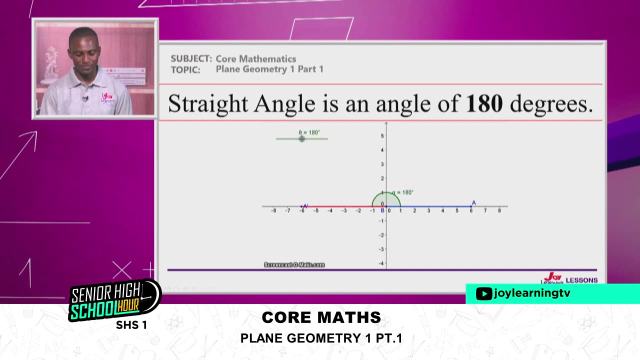 Exactly 90, we call it right angle. After 90, before we get to 180, we call it obtuse angle. What if it falls exactly on the 180 line? Then that becomes a straight angle. So straight angle is an angle of 180 degrees. all right, 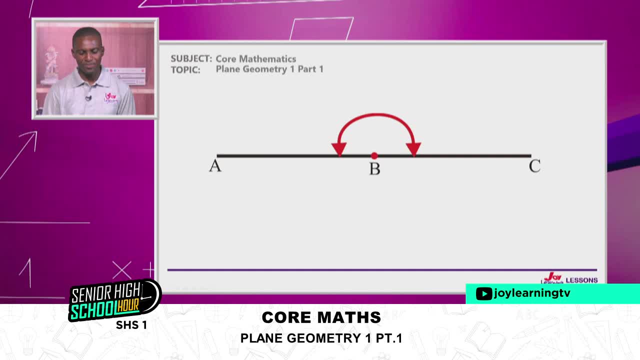 180 degrees beautiful. So again we see angle that forms on a straight line is 180. It doesn't mean a straight line has an angle of 180. Be careful with that. People are making this error. When I draw a straight line, for example, I draw a line segment. 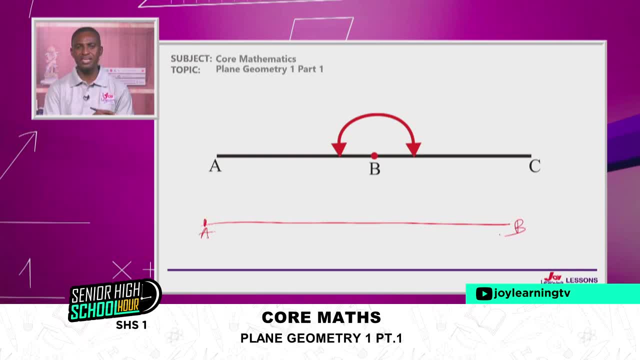 point A and point B. This is just a line segment from A to B, Start from A, ends at B. There's no angle here because I don't have two or more lines meeting. You understand. But the minute I create another point here. 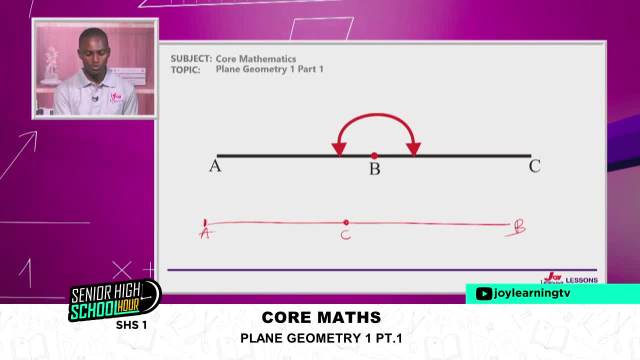 that means that also becomes another line segment, So I can have line segment A C and C B. They are meeting at this point. For that matter, the angle that exists becomes 180.. So angles formed on a straight line makes an angle of 180. 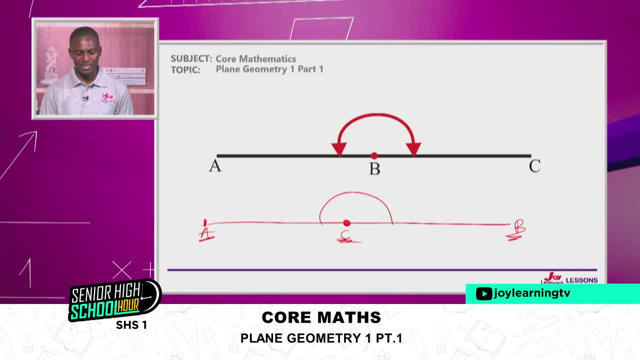 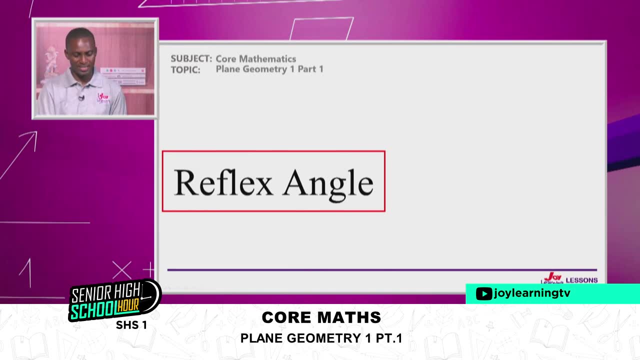 It doesn't mean all straight lines have 180 degrees as an angle. It's not true. Let's be careful when we are trying to define straight angle. Then we go beyond 180.. We go beyond 180, we call it reflex angle. 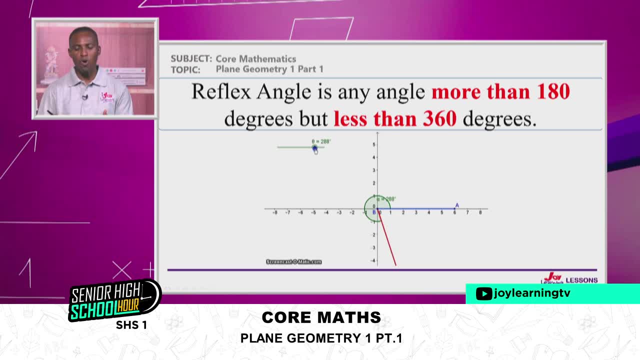 Reflex angle. That means a reflex angle is an angle more than 180 degrees, but less than 360 degrees, So we've traveled beyond 180.. So 270, 280.. 300, 345, 359 degrees, They are all reflex angles. 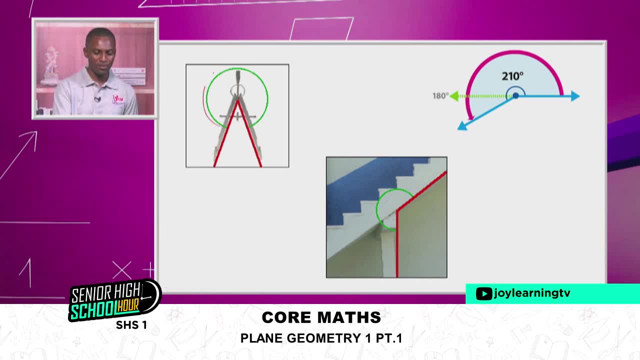 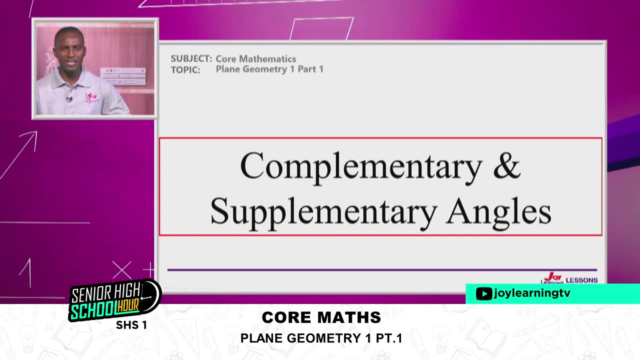 Example can be this: You can see reflex angle here with your compass. You can see it under the staircase here. You can see it over here too as well. I mean, we see reflex angle a lot in our environment. Let's talk about a very important concept as far as angles are concerned. 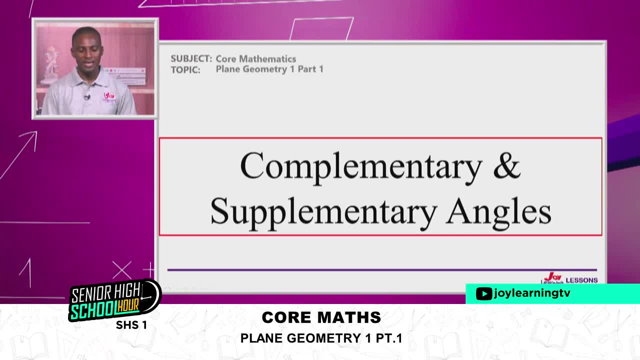 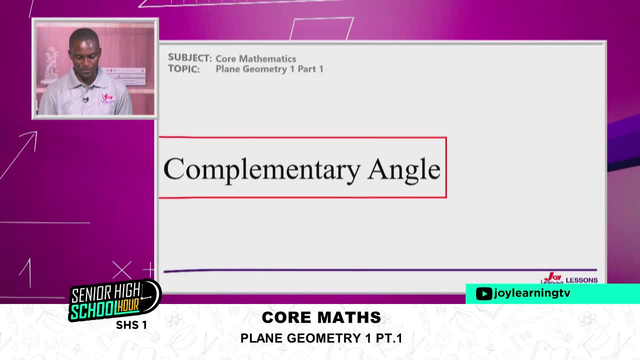 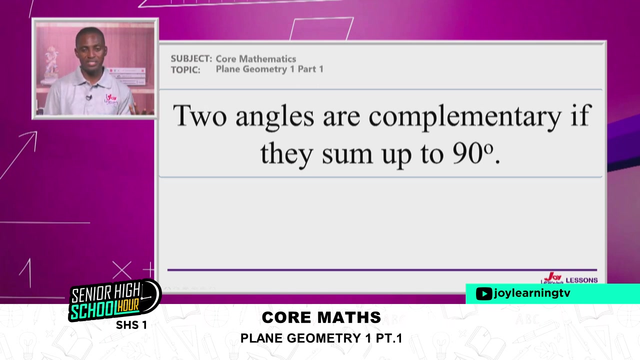 We have what you call complementary angles and supplementary angles. We want to look at what entails into these two concepts here. What are complementary angles? When we say angles are complementary, what does it mean? What does it mean When we pick two angles- 20,, 70,, 20,, 30,, 2,, 5,, 7,, 10,? 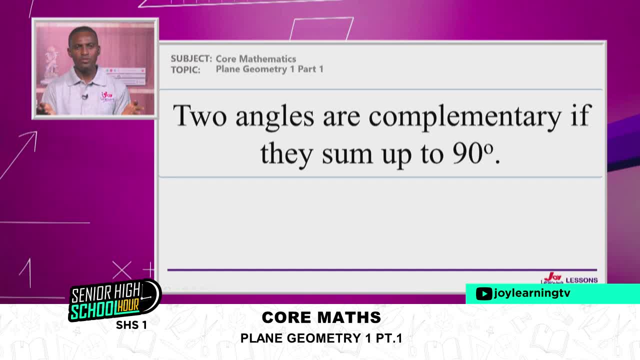 any two angles are all you pick And you bring them together, you sum them and they give you 90 degrees exactly. then those two angles are called complementary angles. So if I pick 70, what will I add to 70 to give me 90?? 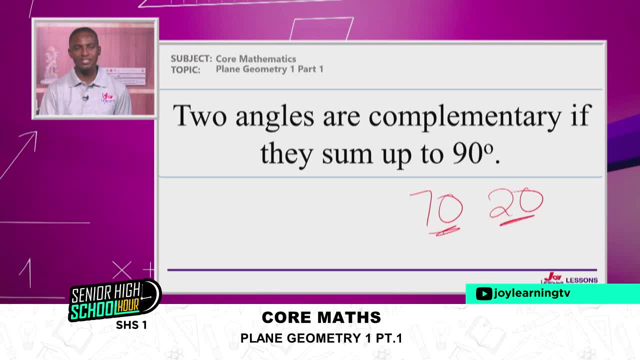 20.. In that case, 70 and 20 are complementary angles. As simple as that, right, Very simple. So 33 degrees, 57 degrees will add up to 90. So they are complementary. Beautiful. Now, if you look at this right-angle triangle here: 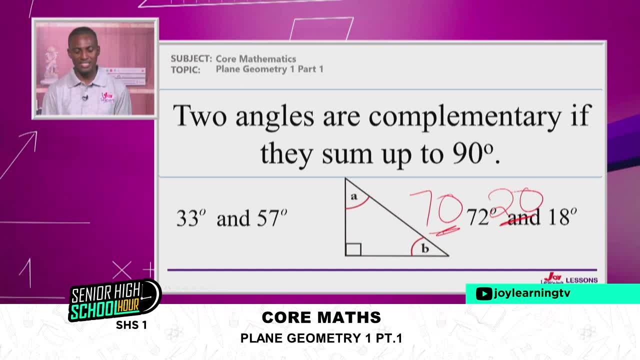 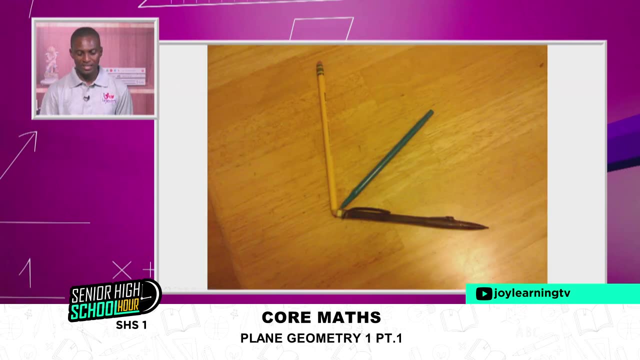 you see that for right-angle triangle, when one angle becomes 90, the remaining two angles must obviously become complementary to each other. So we call them complementary angles. So angle A and B are complementary angles. So here we can see that the two pencils here 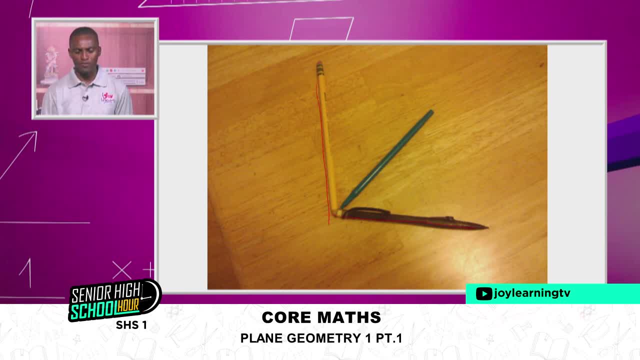 or the pencil yellow and the brown makes an angle of 90. Then we have this green pencil here. Then you can see that the two pencils here we create two different angles And because these two angles will add up to give you 90,. 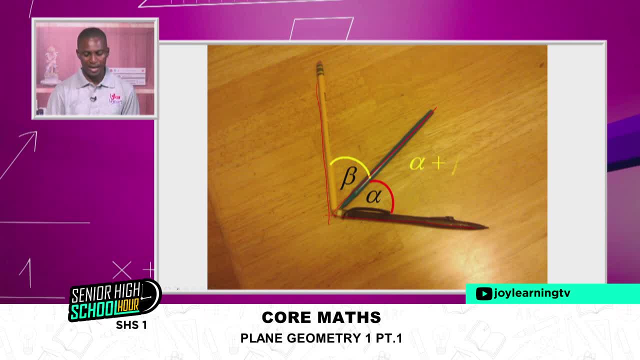 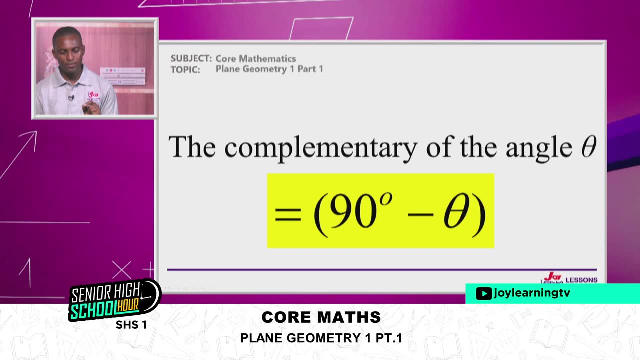 we can say: angle alpha and angle beta are complementary angles, Right? Then again- this is very important because I'm going to give you questions- that you need to use the concept of what I'm going to talk about right now to answer The complementary 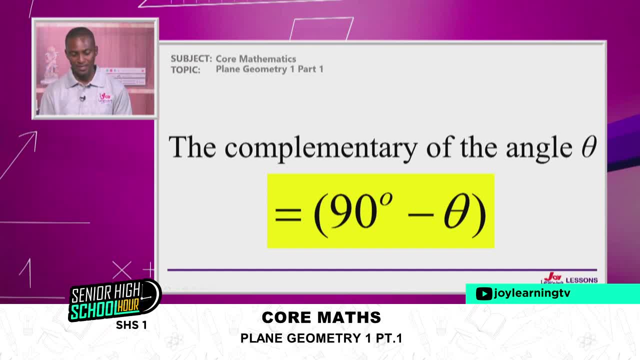 The complementary of The, The angle theta is written as 90 minus theta. What it means is that if I give you an angle, let's say 30, and I ask you what is complementary to angle 30,? what is complementary to angle 30?? 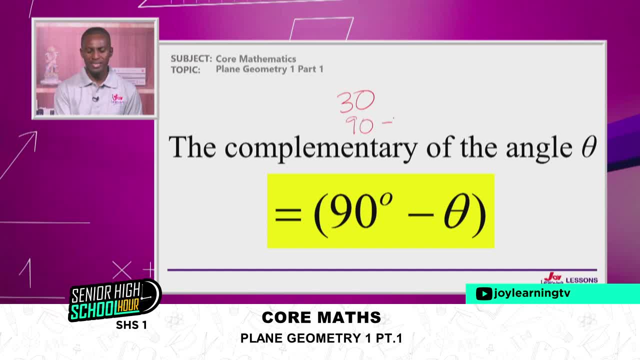 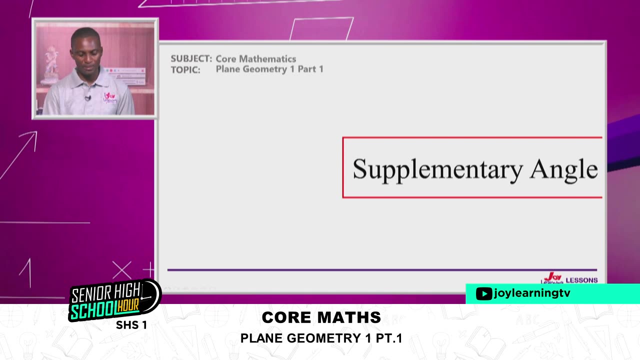 That means I'm asking you: 90 minus 30, what is the answer? You understand? So 60. In that case, 60 and 30 are complementary. They add up to 90 degrees. Then we talk about supplementary angles. 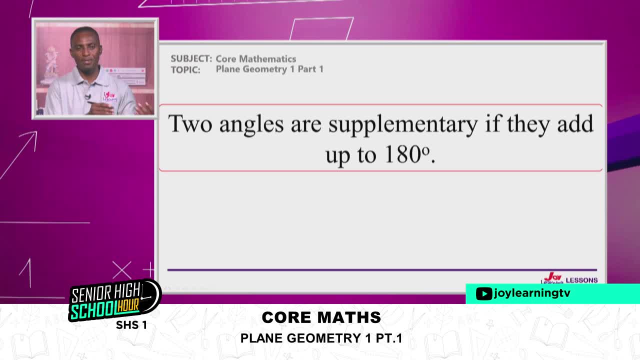 Supplementary angles. And again, whilst we are saying complementary, add up to 90, supplementary also, add up to 180. Example can be 60, 120.. One degree and 179 degrees will give you supplementary angles 82., 98,. they are supplementary. 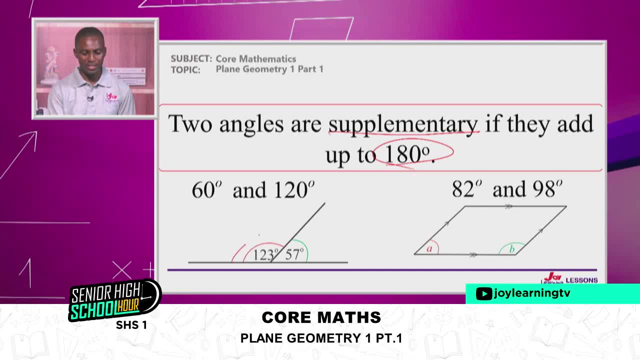 These are supplementary angles. So you can see the form. the two angles are lying on a straight line, having a common vectors, And so we add them up to give you 180.. That means they are supplementary. Now you can see this diagram here, which is a pyrogram. 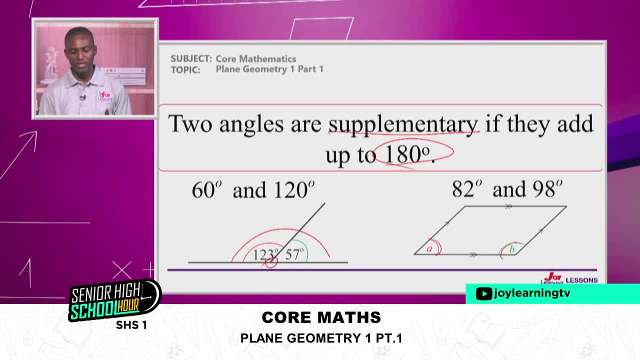 We are saying angle A and B are supplementary because for every pyrogram the consecutive angles always add up to 180.. And so we can say angle A and angle B are supplementary. We'll talk about properties of quadrilaterals in future. You will understand this aspect that I've just mentioned. 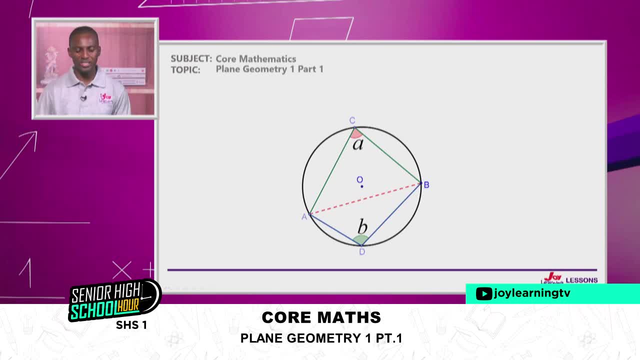 In circle theorem, which I know when you do this topic in year two, when we have a circle and we draw exactly quadrilateral A, B C, so quadrilateral A, D, B C. you see that, You see that. 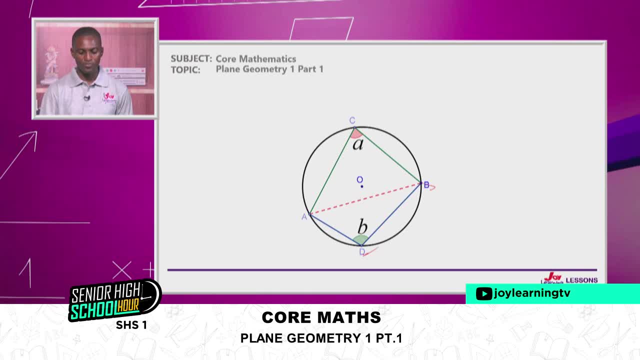 You see that Each of the points touches the circumference of the circle. What we are saying is that opposite angles at opposite segments are always supplementary. I just want to give you examples of supplementary that we see in the course of our work. Now, if an angle is theta, then each supplementary angle ought to be 180 minus theta. 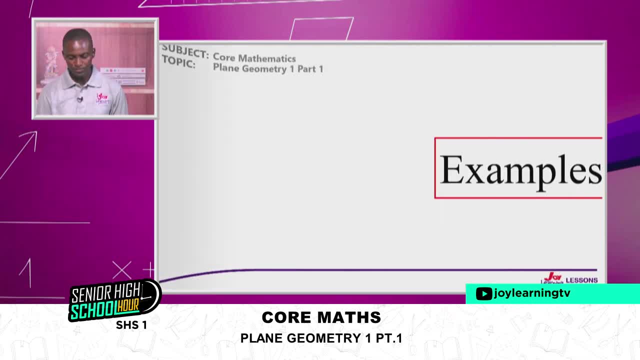 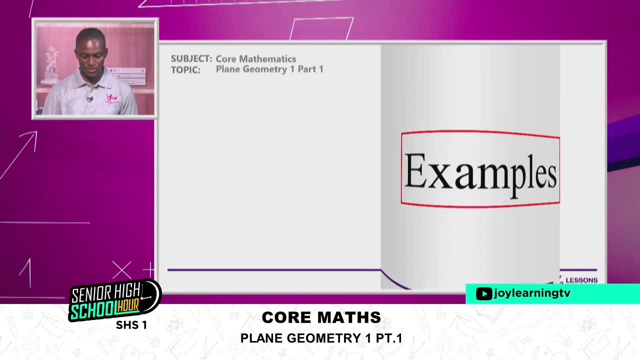 Very important concept to understand as well. Let's take a few questions under what we've done so far. Let's take a few questions under what we've done so far. Let's take a few questions under what we've done so far, Especially with complementary angles. 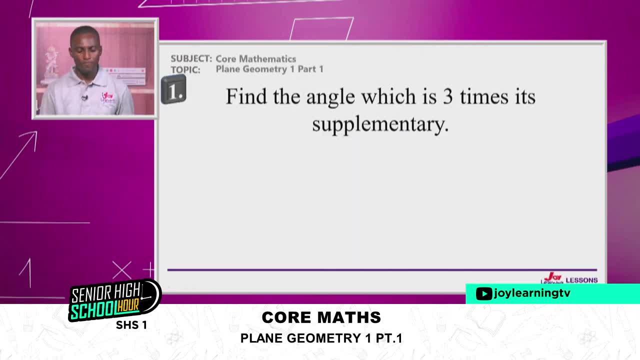 Few examples. I have a question here. Find the angle which is three times eight supplementary. Find the angle which is three times eight supplementary. I don't know the angle, But what I know is that if that angle is, let's say, theta, 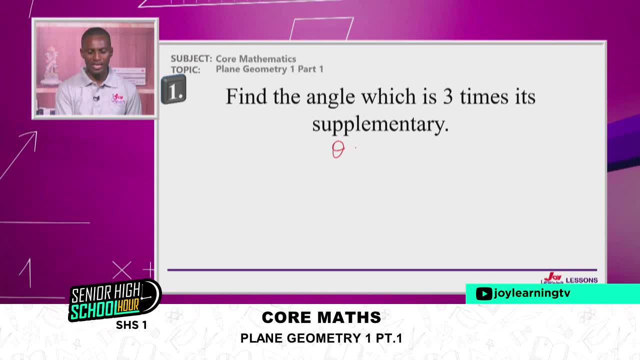 it's three times eight supplementary. So if theta is an angle, then eight supplementary angle would be. but we learned that that's going to give us 180 minus the theta. Okay, And if this theta is equal to three times eight supplementary angle? 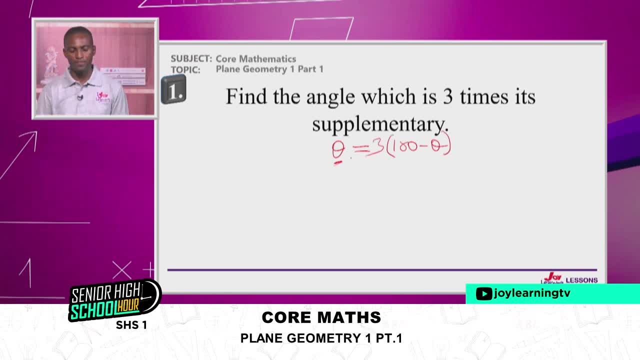 then we are going to have everything multiplied by three here. What is the angle- or what angle are we talking about here- Which has eight supplementary angle three times, And so theta now becomes three times 180 is going to give us Um five, 40, right. 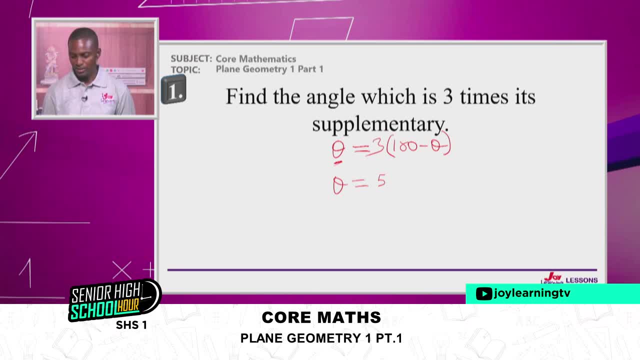 Let me very sure, Sometimes I over- yeah, I think I'm right- Five, 40, then three times um, Tita will give us three Tita. right Again, we want to find a Tita as a subject. 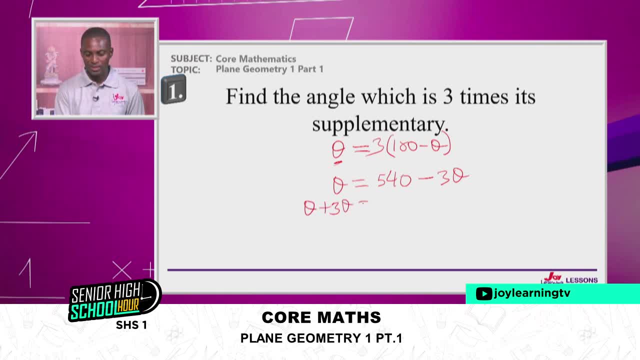 We can group light, And so you have our Tita plus three and the answer will be five, 40 here which we have, this equals five, 40. If it levels are by four, then we can get our Tita to be one, 30, five as the answer. 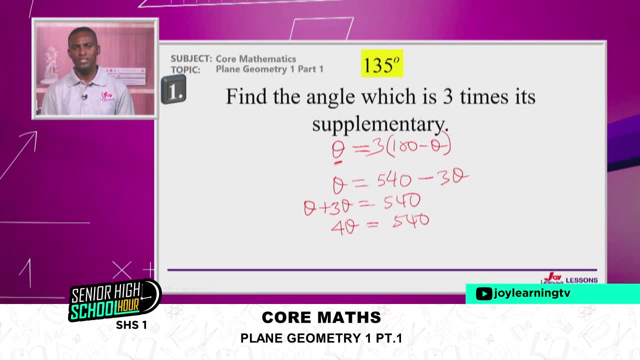 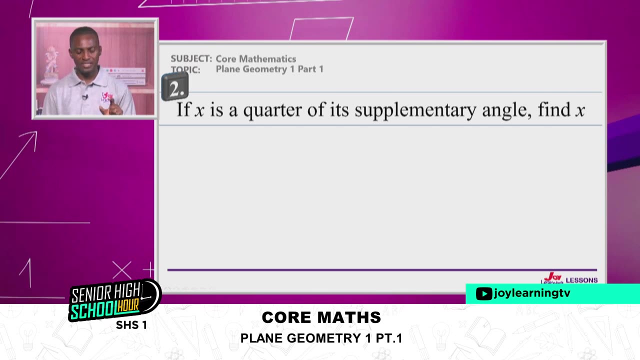 Now these questions comes a lot and you realize that your understanding to the concept of supplementary and complimentary angles helps you solve questions of this sort. Let's take another example and see if X is a quarter angle, a quarter of eight supplementary angle, find the value of X. 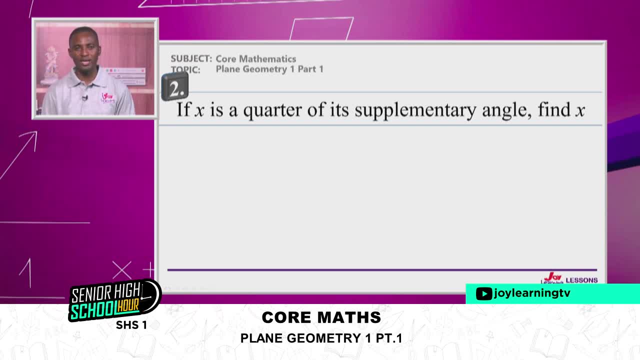 If S is a quarter of eight, supplementary angle: find the value of X. How do we handle this question? If, as a quarter of supplementary, and that means um first of all, if we have X, what is the supplementary angle of X? 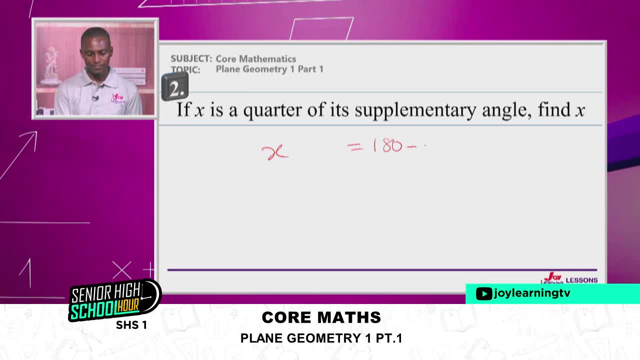 That should give us 180.. My Minus X, right, That is what we've established right now. Oh, sorry. So if X, then the supplementary angle is going to be one 80 minus X. So these two angles must add up to give you one 80,. 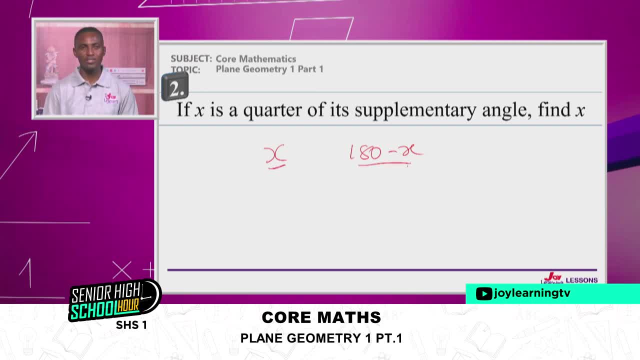 the X and X minus the one, 80 minus S, will add up to give you one 80. They were saying that S is a quarter, a quarter of eight supplementary angle. You see how the language goes: X is a quarter of eight supplementary angle. 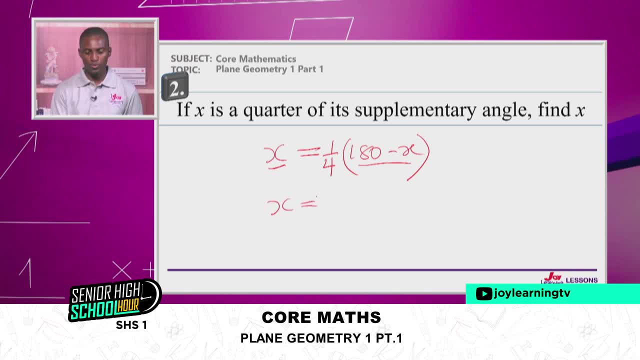 So we can find X Again. if you do um simple cancellation here, we are going to get 45.. That is um. that is one quarter times one, 80.. Okay, It's more, let's say in 180 divided by four. 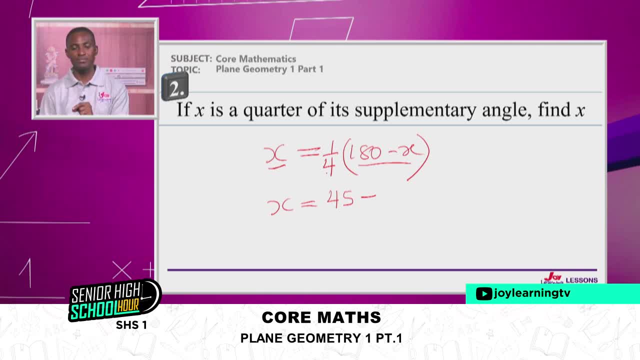 And that will give us 45 minus one quarter times X, And that will give us X on four. Okay, So simple. we can simplify this. actually, from the beginning we could have just say: multiply through by the rcm, so that we get it straight away and say 4x is equal to 180 minus x. but we choose to. 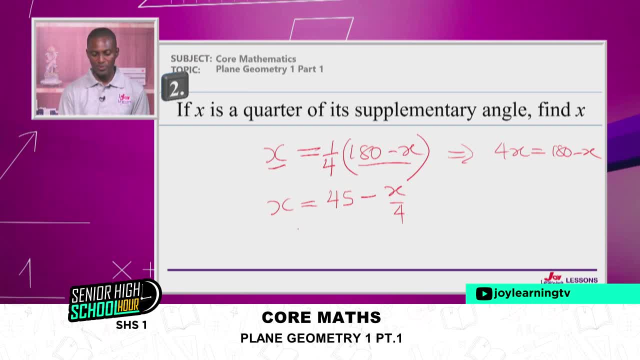 multiply through by 1 over 4, so again it will be the same thing. if i multiply by the rcm, i'm going to get 4x equals 180 minus x. back to that same concept, now making x the subject. so let me ignore this one and work on this. we are going to have 4x- sorry- plus x equals 180 degrees. 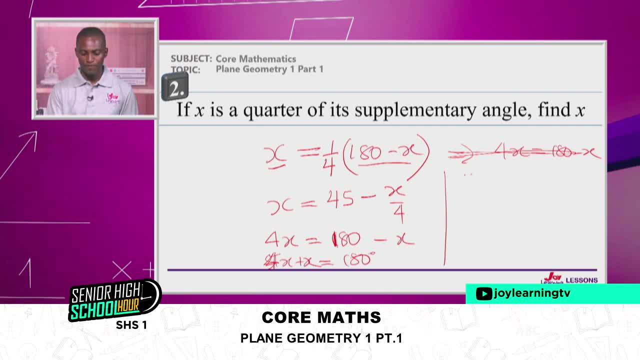 so that will give us: 5x is equal to 180 degrees. divided by 4x equals 180 degrees. divided by 4x equals 180 degrees. dividing both by 5, then we can get our answer to be s being equal to 36. all right. 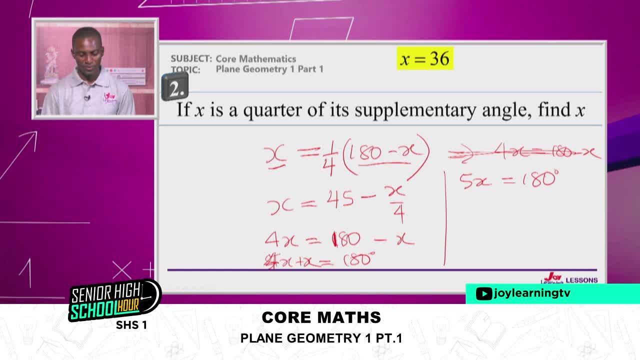 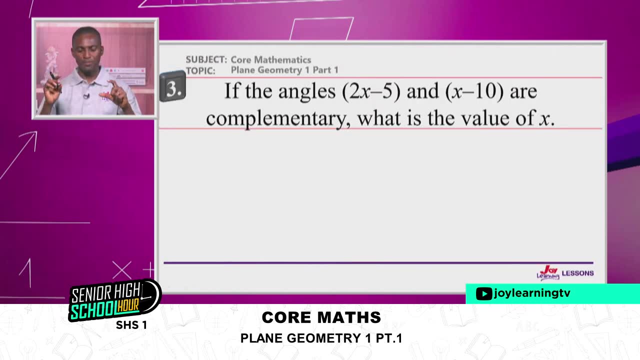 so that is the answer i wish. you can take a picture of this and then solve it on your own. i'll give you the final answer. if the angles 2s minus 5 and x minus 10 are complementary, what is the value of x? if these two angles are complementary, what is the value of? 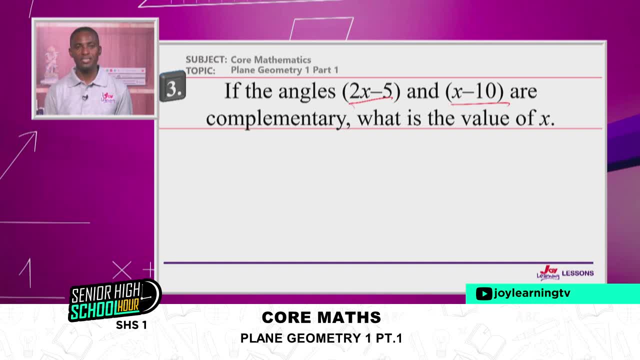 x. if they are complement, what does that mean? it means they sum up to 90.. so if you sum these two, it should be equal to 90, and you can do that and then you get your answer. so when you take your time, you go through it- and i'm sure you do it- and get s to be 35.. 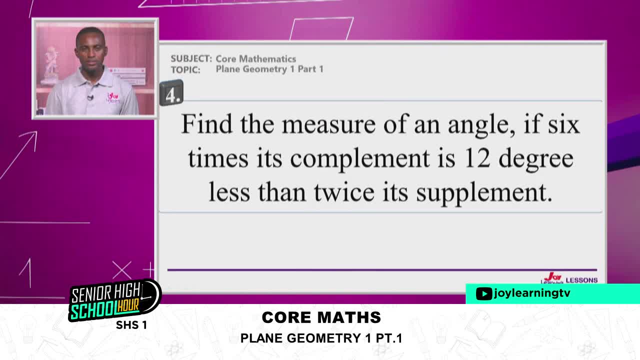 right, take a screenshot of this one too and i'll give you the answer. take your time and work through and see if you can get the answer as such. if you work it well, you get 48 to be the answer. the question says: find the measure of an angle if six times eight complement is 12 degree. 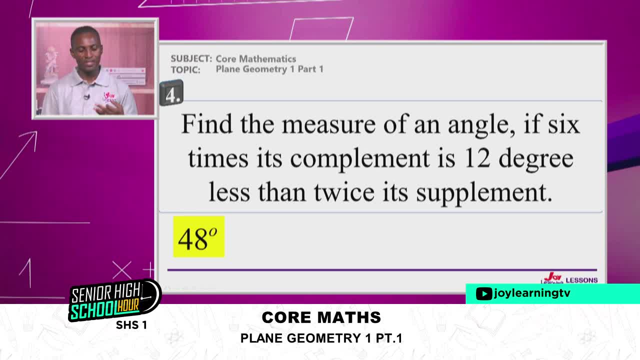 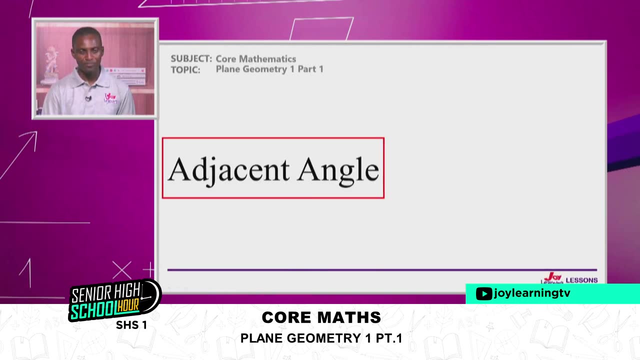 less than twice eight supplement. that means, if the complement angle is six times and that gives you 12 degrees less than eight supplementary angle, what will be the value of that angle? take your time and do this and you get it right now let's talk about adjacent. 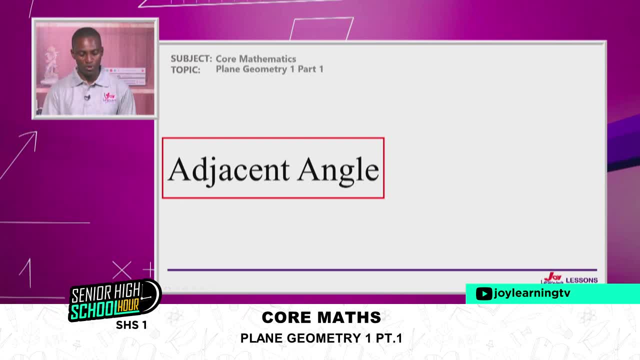 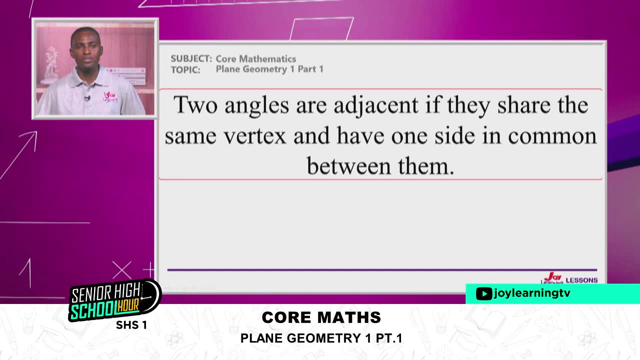 angles, adjacent angles quickly, so that we can do more before our time goes when we think two angles are adjacent. in fact, the word adjacent, we have been using it in our daily life. sometimes we ask people directionally who the house adjacent the? should it be aussihm s a story building? or the house is adjacent the story building? 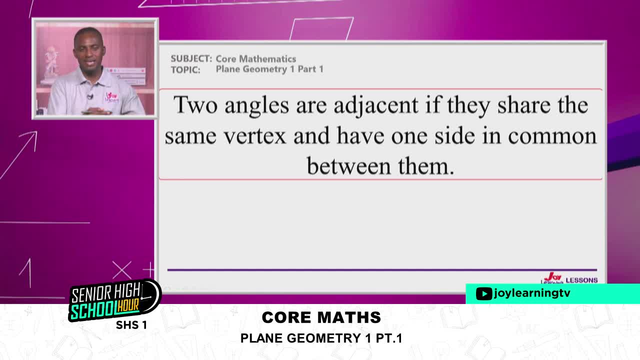 or the house is adjacent, that blue store or blue container, I mean we use it a lot And the way we use it in our daily life. the same thing applies with mathematics as well. So two angles are adjacent if they share the same vectors. 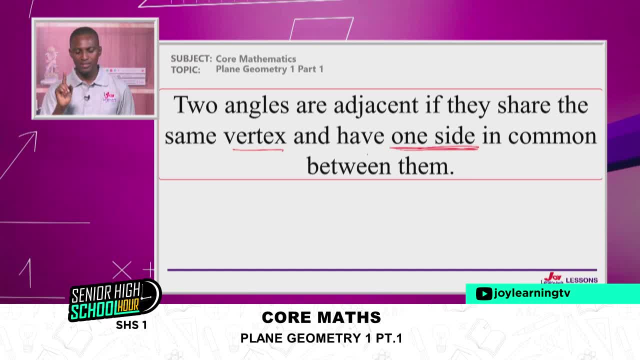 and have one side in common between them. Very important because we need to understand this well. So angle A and B: here we say they are adjacent because they share the same side and they have vectors in common. Then again, look at this: 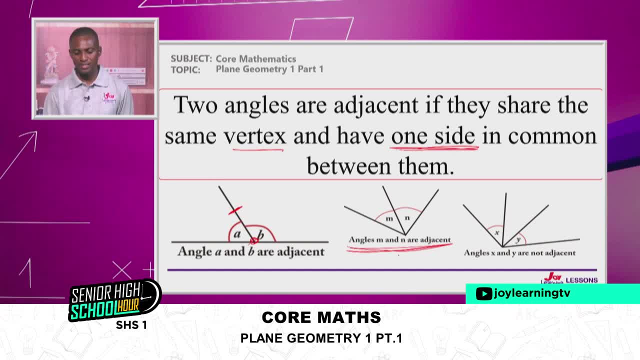 The angle M and N. we say they are adjacent. But look at angle X and Y. Even though they share the same vectors, they don't share the same side or arm, For that matter. we don't want to say that they are adjacent. 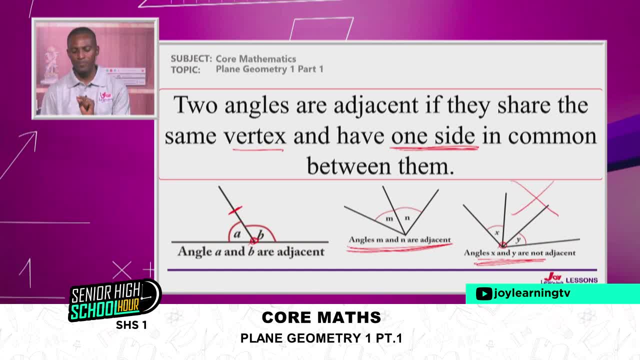 We don't want to say that they are adjacent. We don't call this adjacent angle. So here X and Y are not adjacent, But M and N, A and B are adjacent to each other. Look at this structure. here We can see adjacent angles. 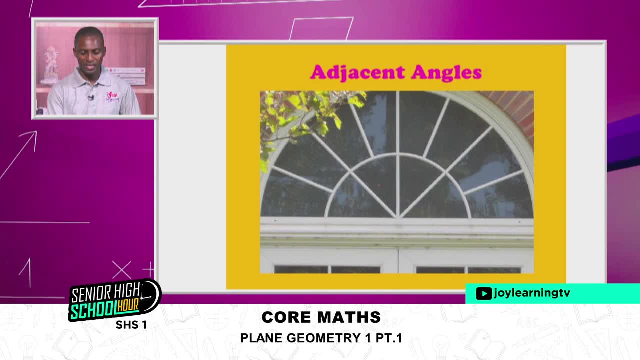 And we use them a lot in our buildings. So you can see that this angle here is adjacent to this angle. Then let's call this angle A, B, C, D. You can see that A, B C are adjacent. B C are adjacent. 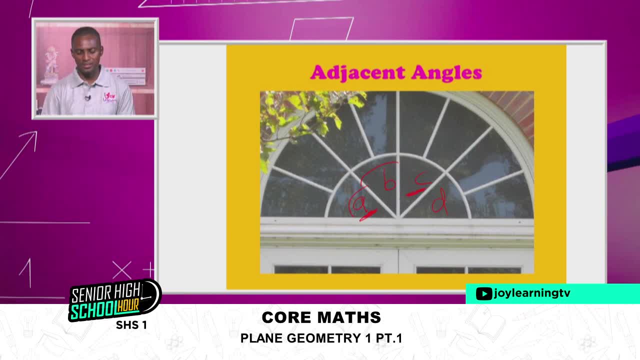 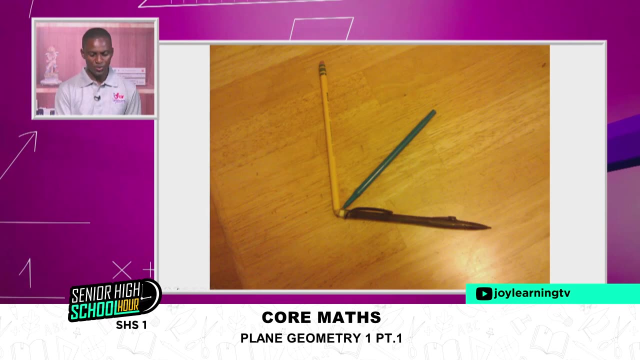 But A and C are not adjacent, C and D are adjacent, B and D are not adjacent. I hope it makes sense. Good, So here can we say they are adjacent angles. here I mean this angle and that angle, are they? 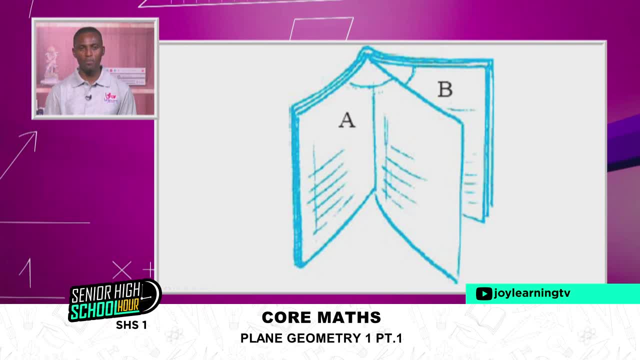 Sure they are. So they are. When you open your book, you also see adjacent angles, right? Yes, So when you open a book, you see that a page can be in the middle, And then we see adjacent angles everywhere. 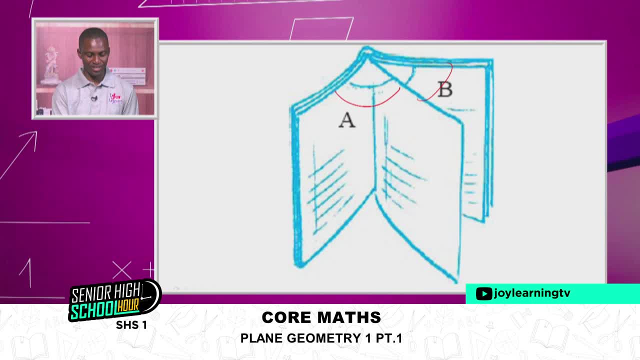 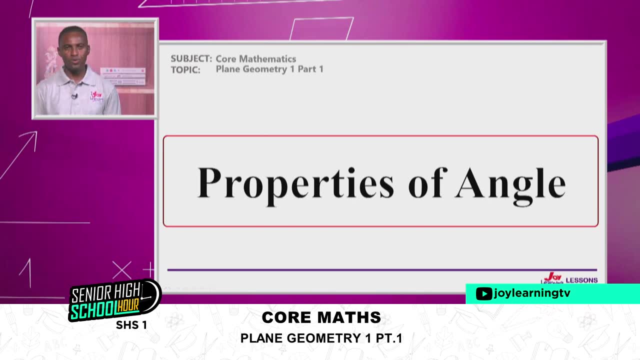 So interesting. Geometry is a very wonderful course for us to study in school because it exposes us to know and understand things around our environment. Now let's conclude this lesson with properties of angles. Properties of angles, And we're going to talk about only a few of them. 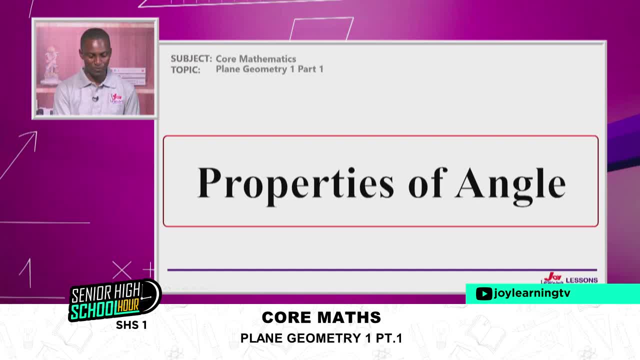 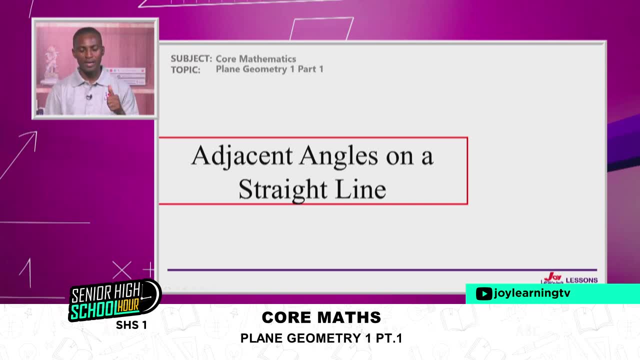 Then our next lesson, that's part two. we'll look at the rest of the properties, So the first one we're going to talk about is adjacent angles on a straight line. Adjacent angles on a straight line. What happens to them if they are on a straight line? 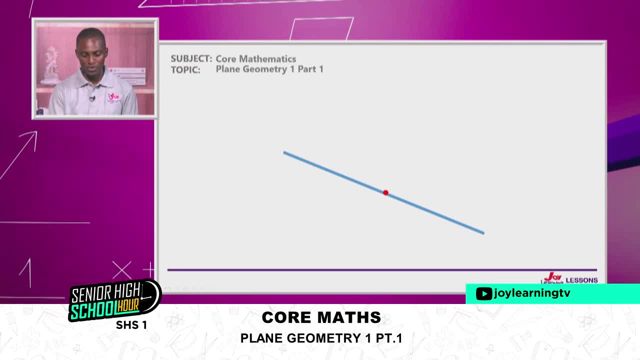 For example, I have these two lines meeting at the point where this red dot is And I create two angles. Call angle A and let's call angle B, Because these two angles are adjacent and they are on the same straight line. we will say they are supplementary. 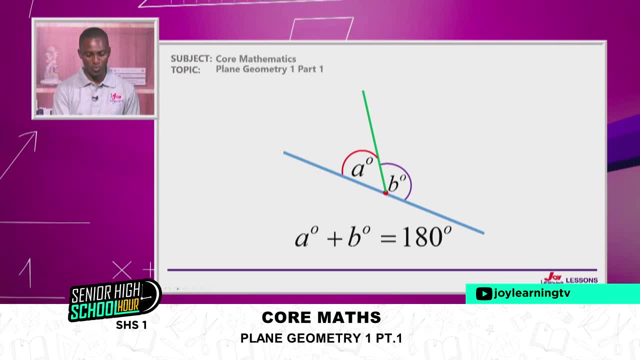 or they add up to 180.. They add up to 180.. Look at these three angles here too: Angles, M, N and R. They all are on the same straight line, sharing the same vectors. It means they add up. to give you supplementary: 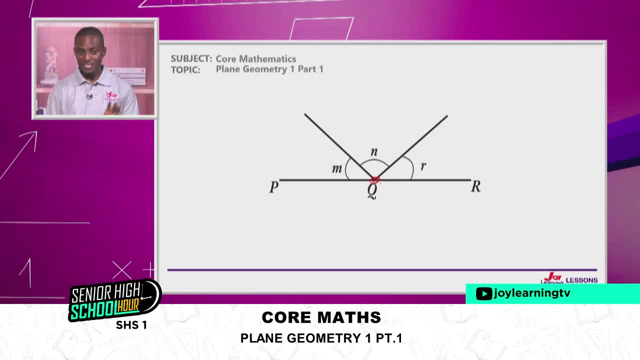 Sorry, they add up to give you 180. But they are not supplementary, Because if they are supplementary it should be only two. So here, even though they add up to 180, we will not say they are supplementary angles No. 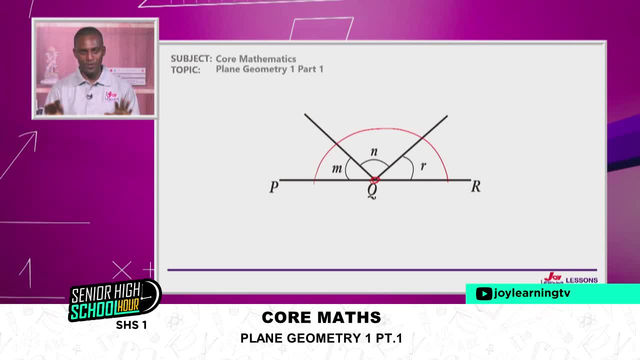 Okay, They only add up to 180, that's fine because they are on the straight line. They only become supplementary if they are only two angles forming or adding up to give you the 180.. Good, So let's take one example or two examples under this. 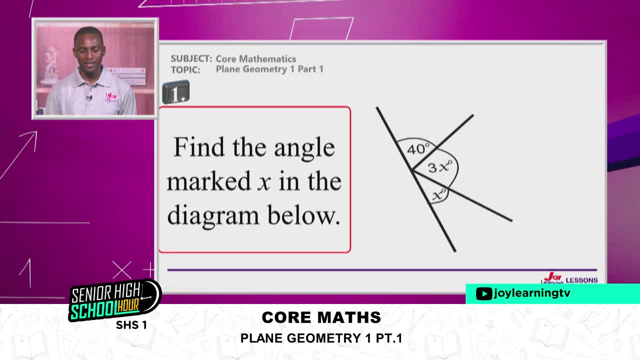 and we'll conclude this part of our course. Find the angle marked X in the diagram below or beside it here. Here is beside, not below. Okay, so how do you find the angle here? Now look at the three angles created here. 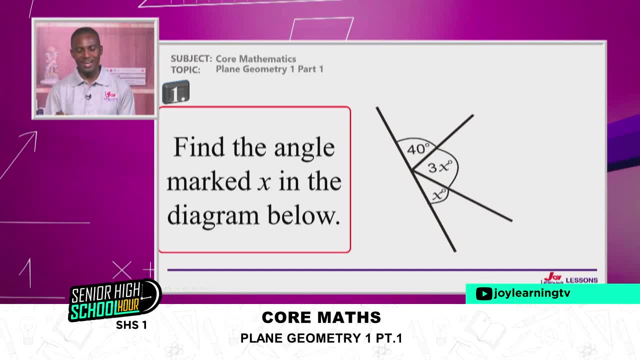 40 degrees, 3X and then X. They are adjacent angles and they are on the same straight line. So we'll say they all add up to give you 180.. So 40 plus 3X plus X, all should give you 180. 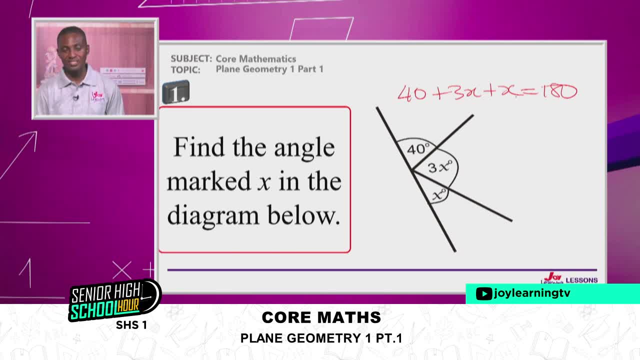 So 40 plus 3X plus X, all should give you 180.. should give you 180 degrees, and solving this is just an algebra. i mean it's very easy, because we've done algebra here, i know you can remember your algebra. so this will give you 40 plus 4x. 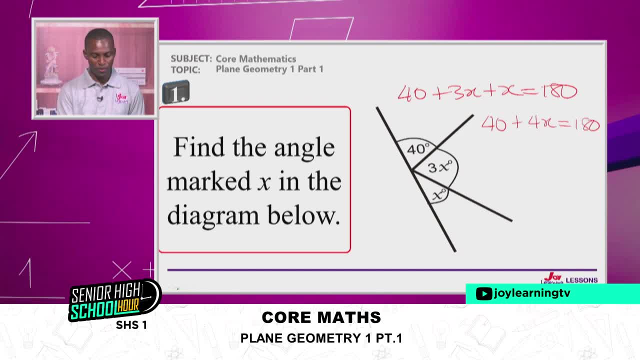 equals 180.. if you do the calculation very well, you get your answer to be 35 as x. now let me let me make something clear here before we continue. if i have this angle x and i have this angle y, the two angles are on a straight line, but they don't share the same. 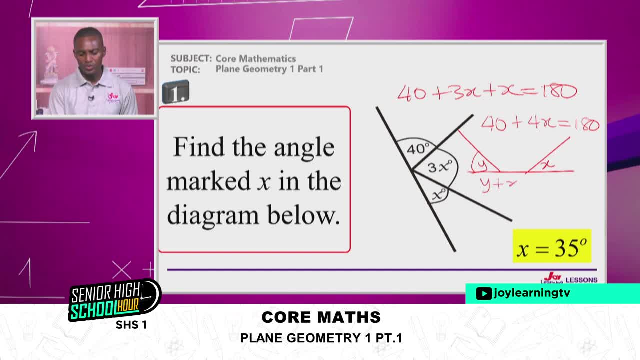 vectors so we can see y plus s will add up to 180.. so let's make this error a lot. so let's be very careful when we see angles on a straight line, even though dsd on the on the straight line, the two of them are on the same line but they don't have the same vectors and so we can't see the. 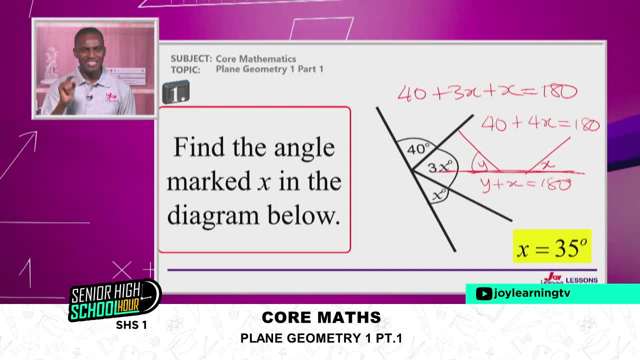 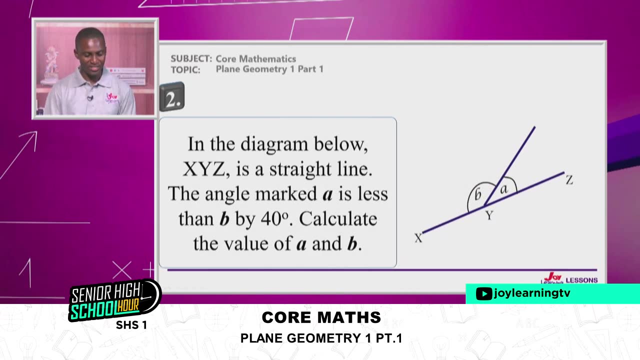 adjacent angle is the straight line and, moreover, they are not adjacent in the first place? yes, because they don't share the same side. okay, beautiful. so let's be careful about that. now look at this question here, which will be our last question to end this section. then i'll give you a size to do. in the diagram below, xyz is a straight. 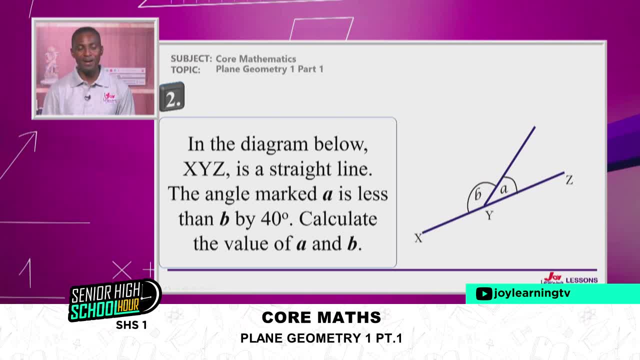 line. the angle marked a is less than b by 40. find the value of a and b. find the value of a and b. so maybe we know. first of all, they add up to 180. that's the first and foremost thing. then we are saying that the angle marked a is less than b by 40. so a is less than b by 40. that means b minus. 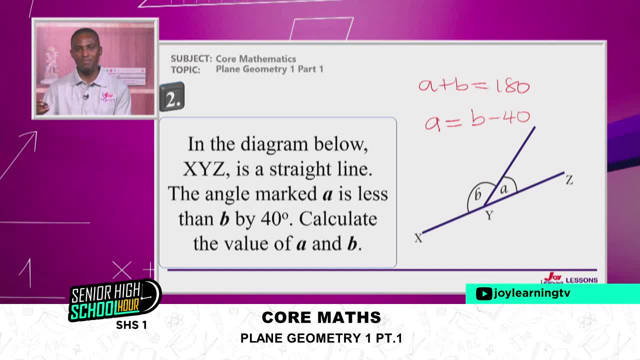 40. so a can be equal to b, but then it must be less than 40 before it will be equal, and if that is true, then we have a plus b equals this of a. i can put this over there, right, so that i have b. so instead of a i'll have b minus 40. 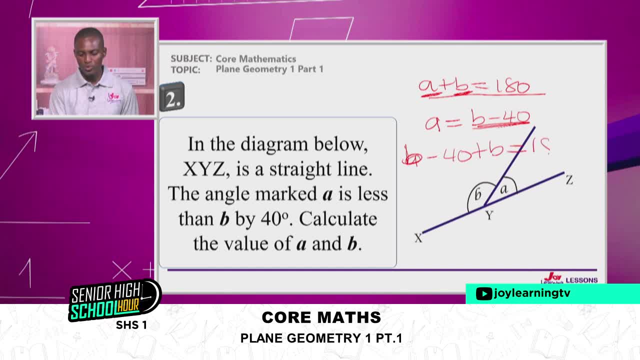 then plus b is equals to 180. then we can make b the subject right. so you have: 2b is equals to um 180 plus 40. and if you add 180 plus 40 you get to um 20.. divide both side by 2 and that will. 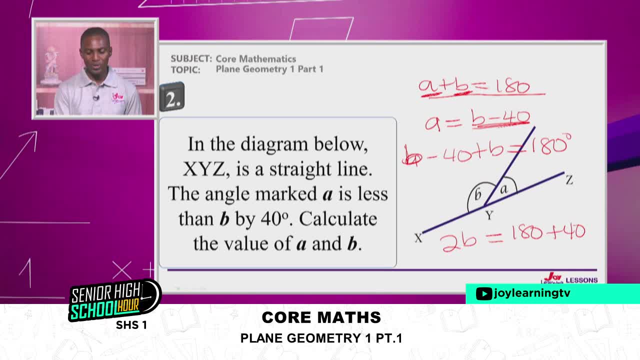 give you b to be 110, and if b is 110, then you can easily know your a, because if you put 110 in place of b, you can make a the subject and a will give you 70 was b is 110, as we said. so let's conclude. 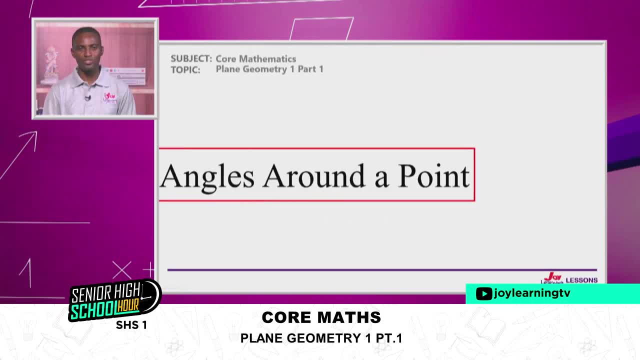 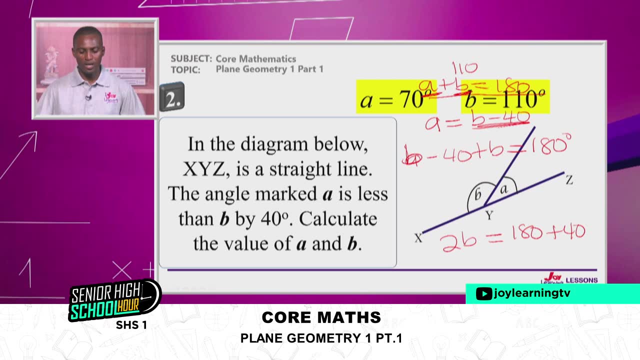 by. oh, i thought about it going to give you this snap question to do, but i don't have time to do that. so what have you learned so far? this has been the shsr for um on joint learning, and then we are dealing with core mathematics, and the topic has been plain geometry one. 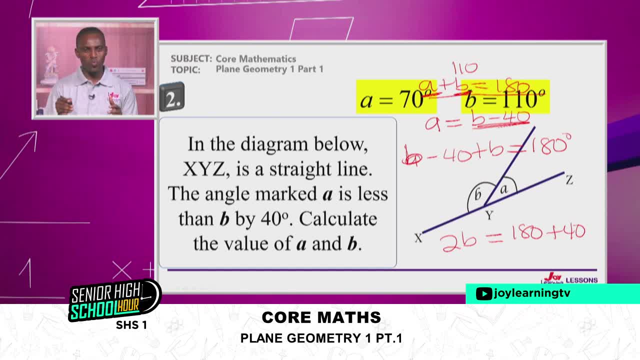 it means you have plain geometry two, but then with plain geometry one we are dealing with part one, because we have a lot of concept to learn in part in plain geometry. so we've went through three fundamental uh terms like line, plane and point, and based on these three terms, 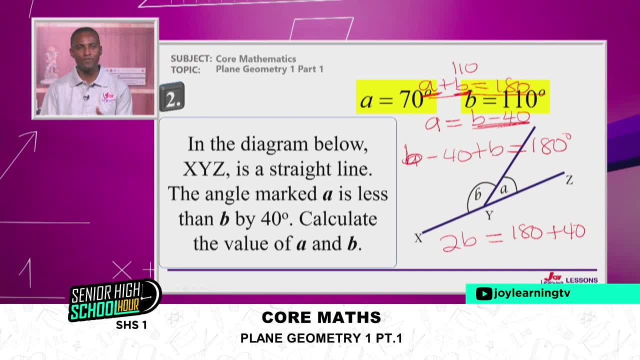 you can define all other terms. so we first defined angles and we've been working with angles. all this while we've said about types of angles, we have acute obtuse reflex, a right angle and straight angle. it will talk about complementary and supplementary angle. they will talk about angles forming on a straight line. that is the file we've been able to go for. 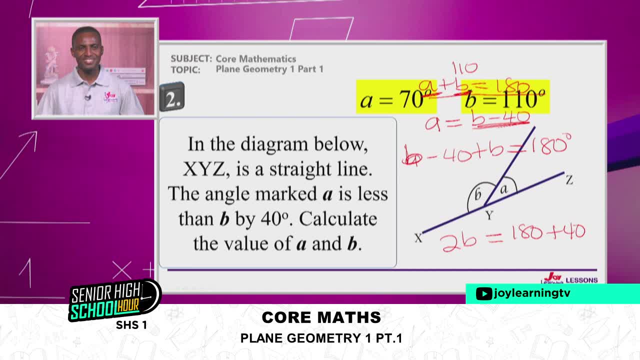 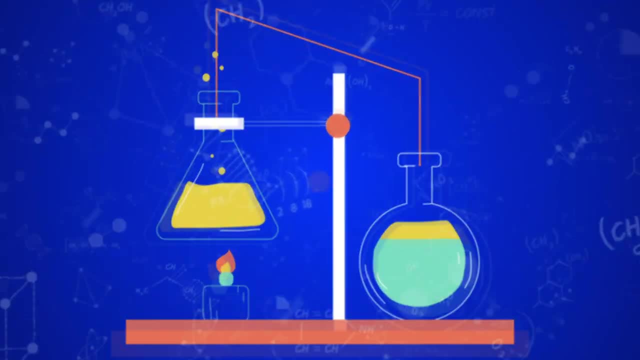 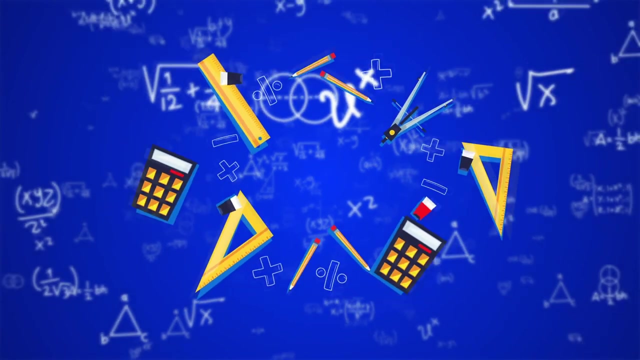 today. i'm sure you've learned a lot and this has been your facilitator events all day. thanks so much for watching. see you another time for part two of this lesson. bye-bye. subscribe to our youtube channel: joy learning tv.